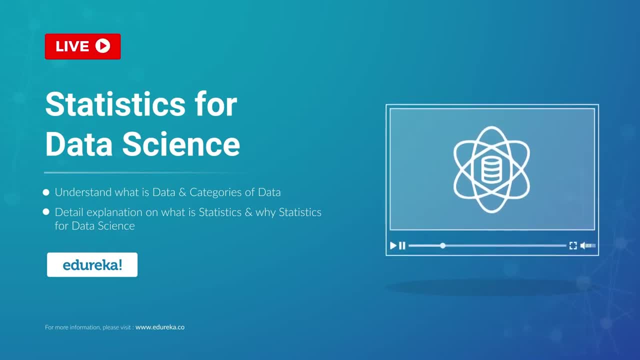 deviation variance, kurtosis, p-value, z-score. A lot of statistics have been involved in all these algorithms, like linear regression, logistic regression, decision quiz, random forest, nav-based classifier. All these algorithms are very popular And all these algorithms 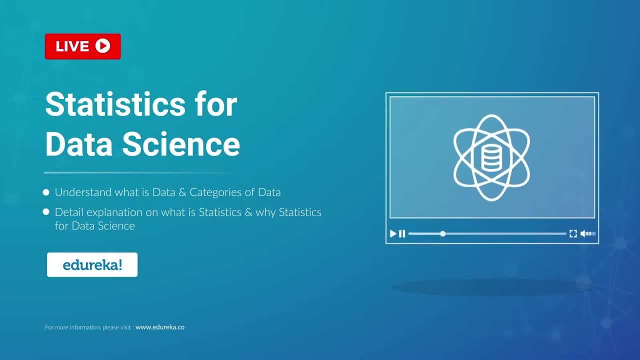 are statistically driven in the back end. So that is the reason machine learning is very popular And stats is the backbone of it. If you are good in stats, if you are good in fundamentals of stats, I will not say that you need to have a graduation knowledge of 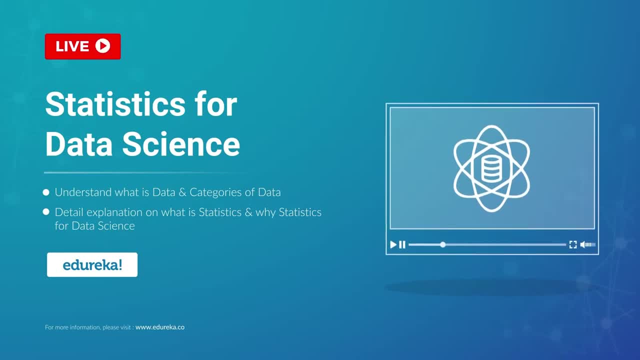 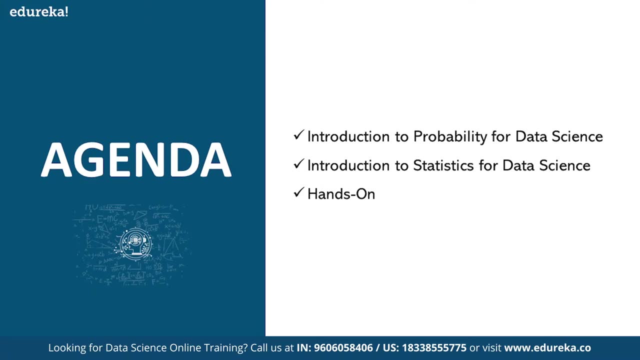 statistics. But fundamentally, if you are good in basic statistics, you can work very well in machine learning algorithms. Now agenda for today's session is we will talk about introduction to probability of our data science, introduction to stats for data science and maybe some 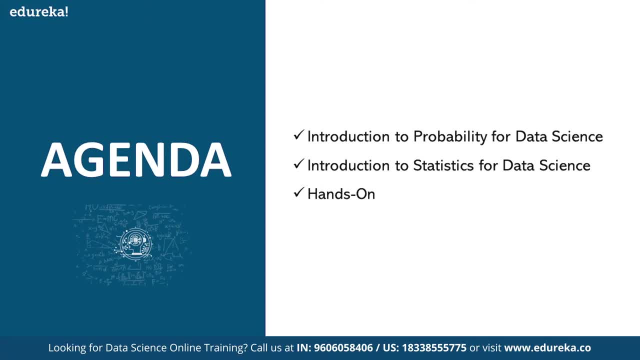 things you can learn about data science. So let's get started. I will be starting with a demo of how to easily find the solutions using python built-in functions. I don't know how many of you do not know Python side, But I can show you some demos on the. 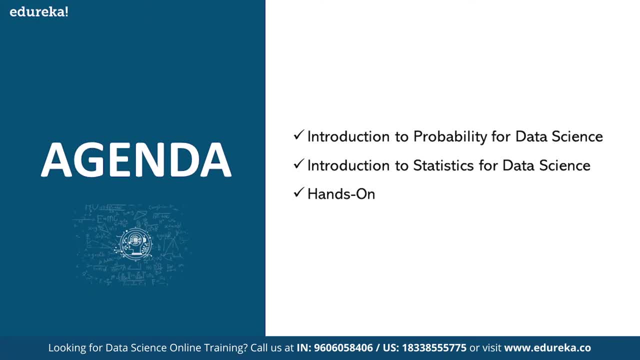 Python side How to easily find the solutions using Python inbuilt functions, where you can use it and you don't have to reinvent the wheel. You don't have to learn the statistical formula for any kind of a scenario. You just need to pass the function and pass the value. 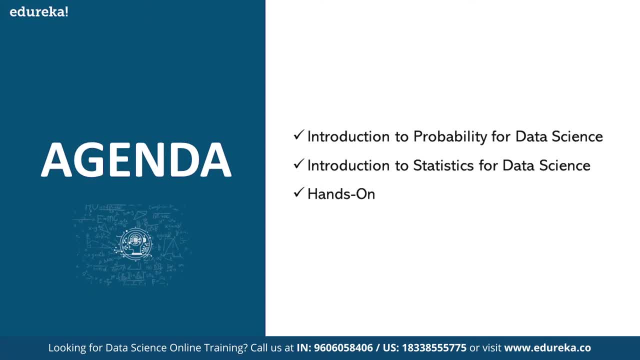 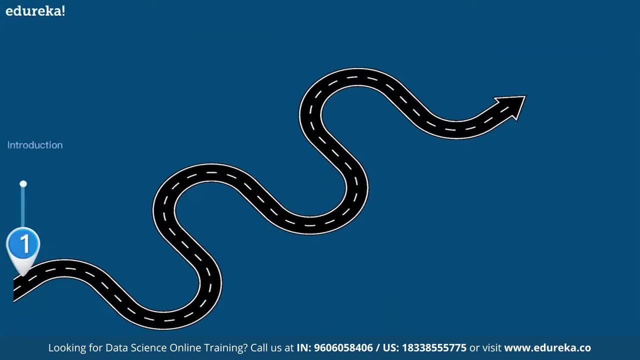 into it and you will get the results in one line. Now, if we talk about a road map for a data science, first and foremost thing is you need to understand and do the hands-on on python. so python is a very popular programming language. maybe python or r. i would suggest python because 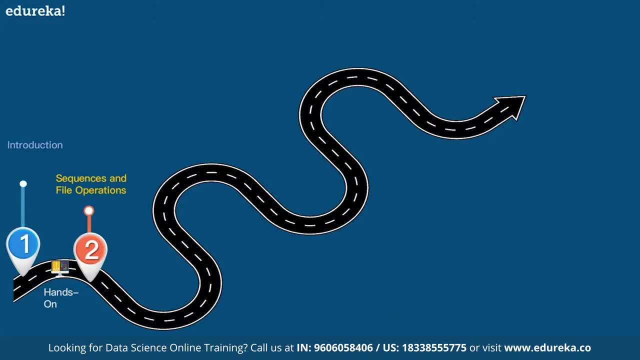 python is a king of all the programming languages and r is called as a golden child of programming languages. so you need to be very good in python. in python there's a topic called sequence and file operations. sequence means list, tuples, dictionaries and how to handle the external files. then you need 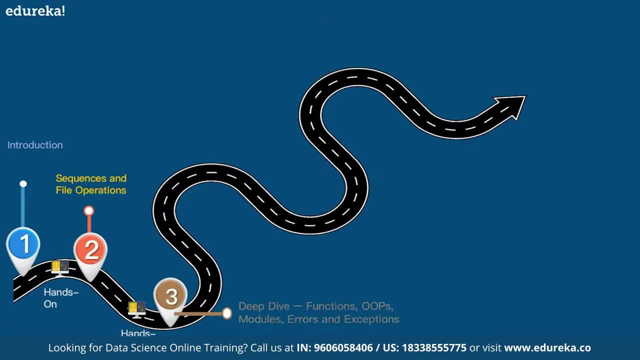 to work on functions, object-oriented programming, programming modules, inbuilt modules, error and exception handling. so modules are nothing but the header files which you include on top of our code. for example, if you include in the top of the code math dot math, you can use all the functions of 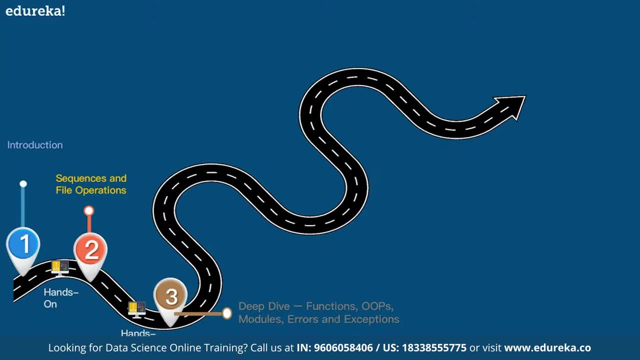 math like square root, like factorial, like cosine value, sine value, tan value. so modules are nothing but the header files which you include on top of our code, which you can reuse to get the work done in a easy way. so these are the important things that you need to know. after that you have section to numpy pandas on matplotlib. so these are three important. 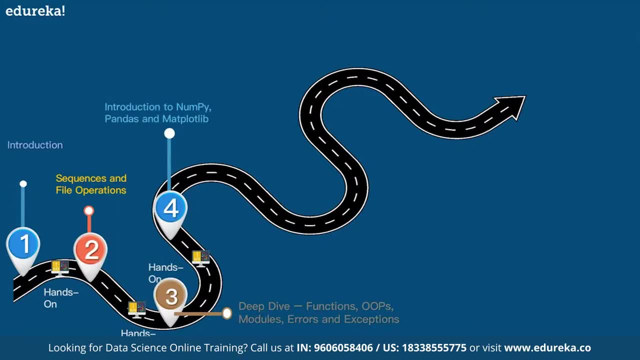 libraries in python which is primarily used for data analytics, like numpy is for numerical analysis. suppose you want to find standard deviation. you want to find any statistical inference, like covex, variance, variance, kurtosis, p-value, z-score, Anything you want to find statistically. 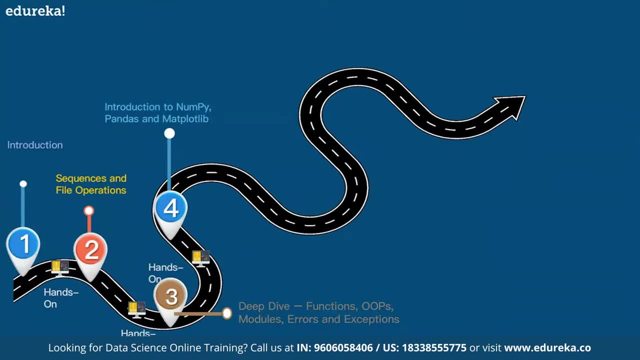 can be seen from NumPy library. Panda is a library for data analytics. Suppose you want to do data wrangling like data munging, cleaning, joining, concatenating, filtering, subsetting, writing down some complex queries on the data, doing some statistical inference on the data. 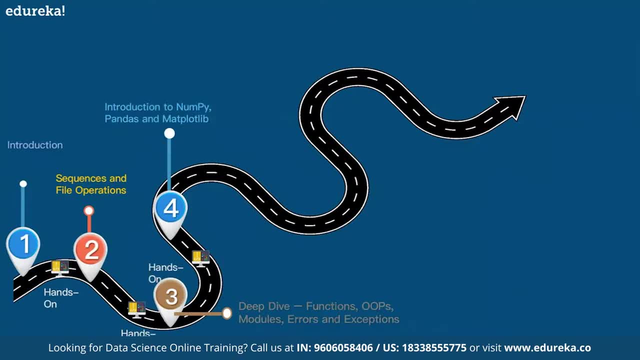 So Pandas can read the data from any external file And Matplotlib is a library in Python for plotting graphs. Suppose you want to plot a histogram or a pie chart or a scatter plot or any kind of a graph, line graph. 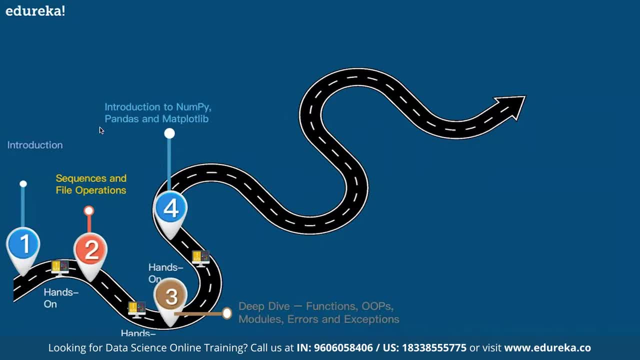 then you use Matplotlib. So NumPy is for the microanalysis, Panda is for data analytics, Matplotlib is for plotting graphs in Python. So you need to be very good in this area, because most of the data which you come across will be not clean. 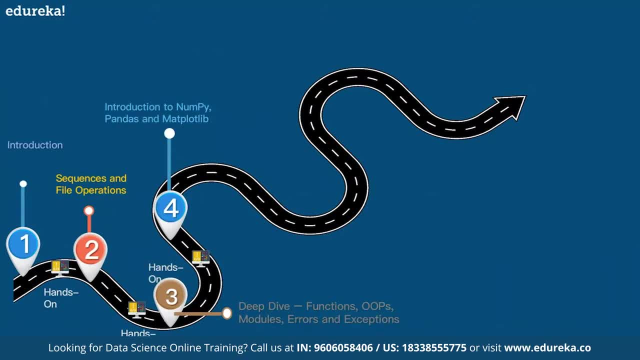 Not clean means it may have a lot of outliers, It may have missing values, It may have dollar symbols, It may have special characters, It may have unclean data there in it. So you need to remove some rows, You need to remove some columns. 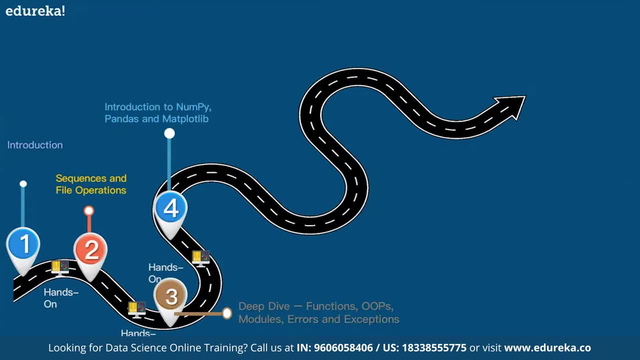 You need to join that data with some other data And do a lot of data wrangling and visualization before going for machine learning. So machine learning is the last step, where you do predictive analytics And then comes data manipulation using all this NumPy Pandas and Matplotlib. 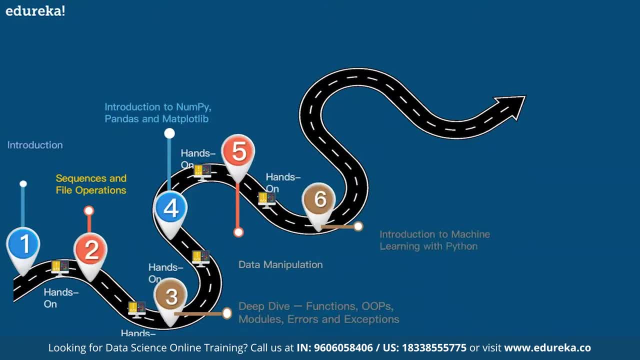 And then comes introduction to machine learning, where we have three types of machine learning: supervised, unsupervised and reinforced. Unsupervised means where you know the column headings completely Unsupervised means where you do not know the column headings and we use clustering algorithms. 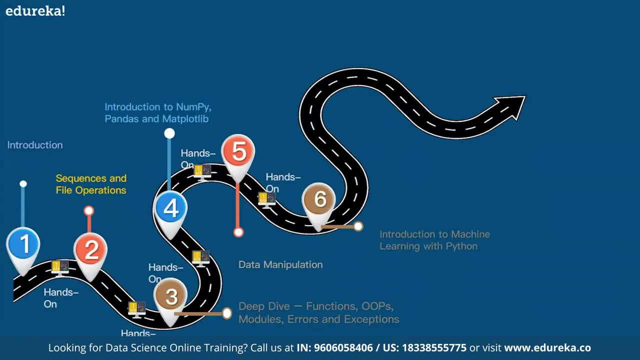 Reinforcement learning is learning with experience, slow and gradual learning. So machine learning is a last part in terms of learning Python, learning stats learning, data analytics, and then comes machine learning, And then comes dimensionality reduction. Suppose the number of features, number of columns. 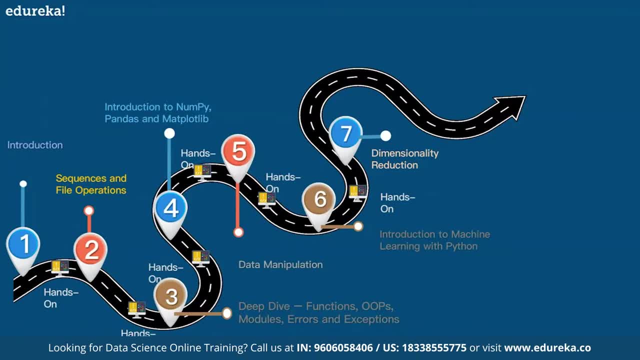 in your data is quite large. you want to reduce it. You want to reduce it to lesser number of columns. There's an algorithm in Python called PCNLDA- principal component analysis and linear discriminant analysis- by which you can reduce the data into a smaller size. 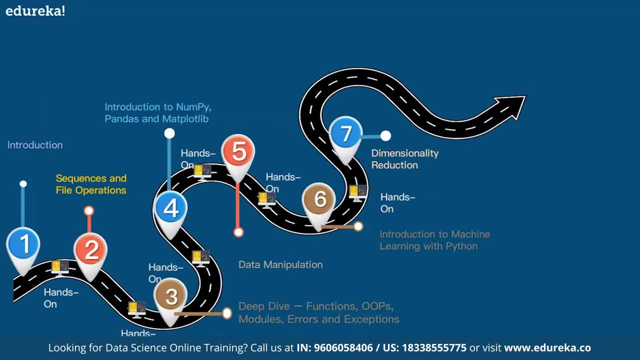 so that your machine learning algorithm will run faster. Dimensionality reduction is an important topic which you need to learn. Then comes the unsupervised machine learning, where clustering algorithm happens like K-means clustering, C-means clustering, agglomerative clustering. 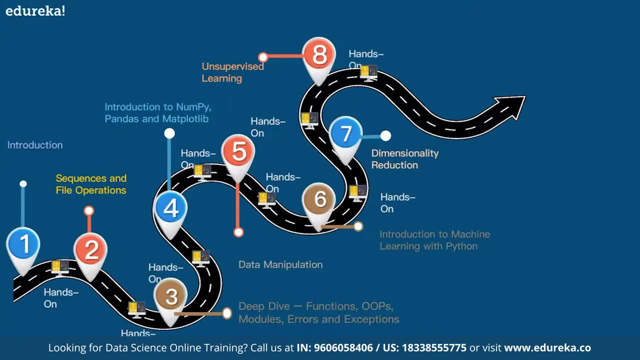 All the clustering algorithms comes under unsupervised machine learning And finally you get a after doing association rule and recommendation engines. Association rule means how one product is related to another and recommendation engine is: after buying something, system is recommending you to buy some other thing. 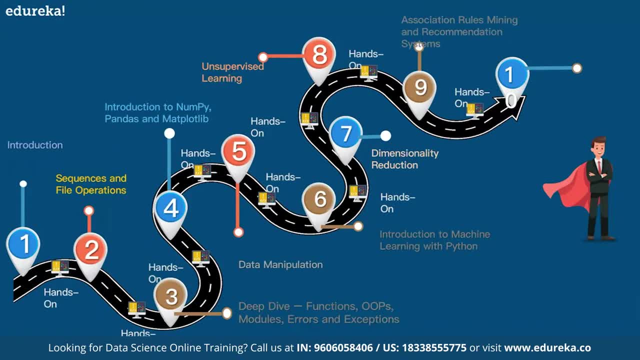 Suppose you go to Netflix and watch thriller movies. So Netflix recommends you. why don't you watch another thriller movie? So that is again a machine learning part. And then finally comes the reinforcement learning, that is, learning with experience and slow and gradual learning. 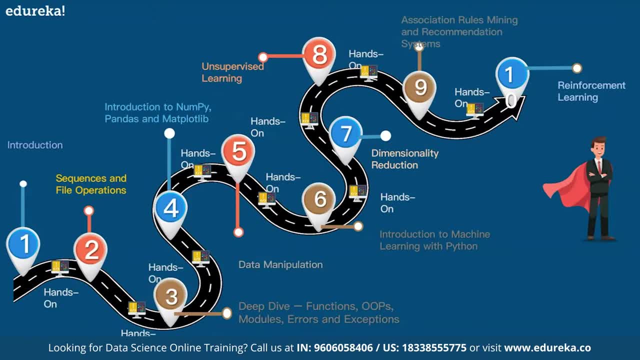 So this is the complete roadmap, slow and gradual roadmap for a person maybe experienced in programming, maybe not experienced, but it is a value add if you already know some other programming languages like C, C++, Java, But it's sort of prerequisite. 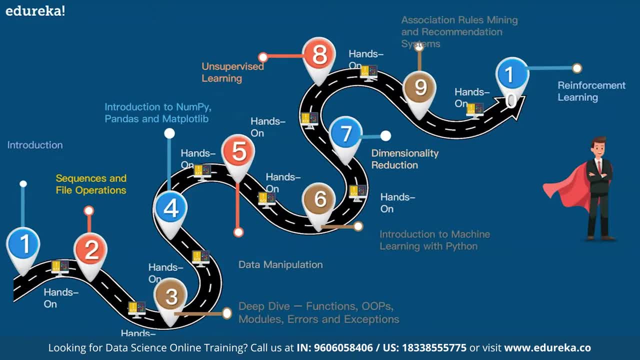 anyone from the non-IT background can also learn this. Only thing is that a lot of hands-on and practice is required, And this is a roadmap for a complete data science, where we start from the beginning, from fundamentals of Python, and slowly and gradually move towards. 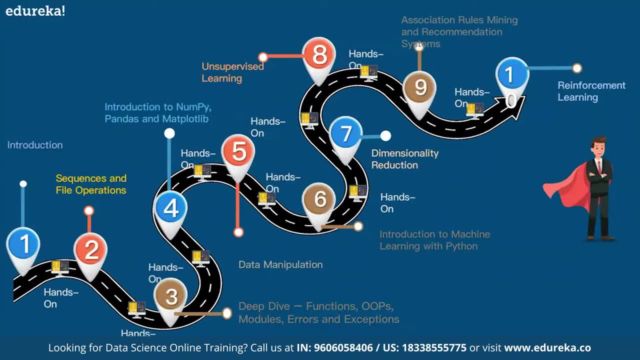 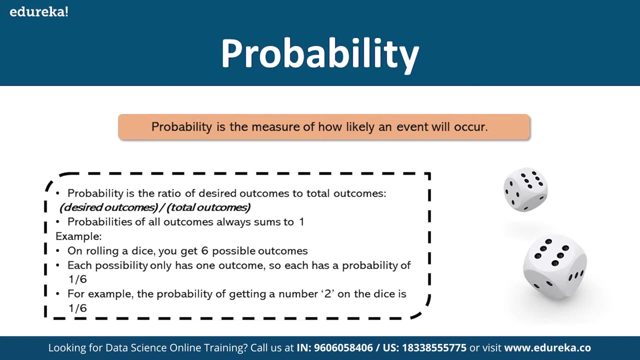 data analytics and then move on to machine learning, and after that there is another part that is called deep learning, which is a subset of machine learning. once you complete all this, then comes deep learning. now let's quickly talk about probability, most of the things we already know. this is up till 10th standard of mathematics. we have learned all this, so probability is nothing. 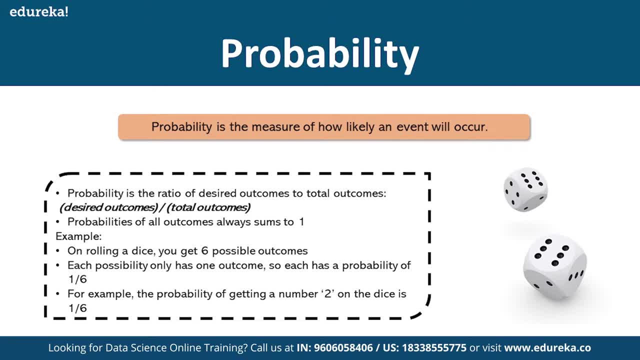 but the ratio of desired outcomes out of total outcomes. so what we are desiring out of total outcomes is just a probability. probability is always sums it to one. so if you sum all the probability values of all the events, it will come out to be one. for example, rolling a dice, you get 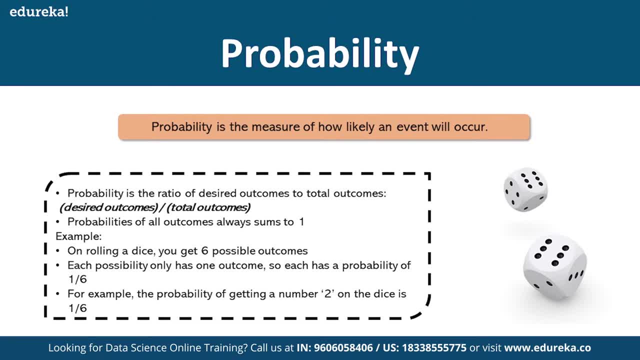 six possible outcomes. so probability of each outcome is one by six. the probability of getting one is one by six. probability of getting two on the dice is one by six. again, the probability of getting each number of the dice is one by six. so that is probability, like what is the. 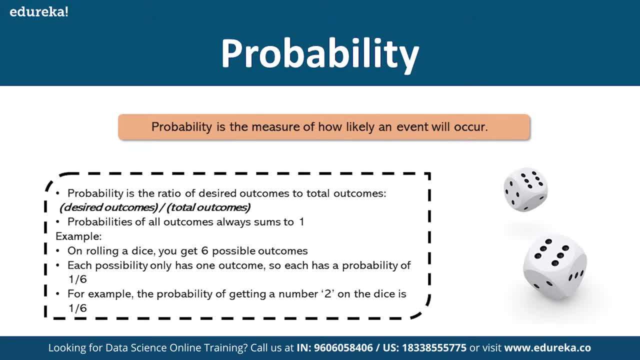 likelihood of getting two on the dice is one by six. so that is probability. like what is? the likelihood of getting two on the dice is one by six. so that is probability. like what is the likelihood of getting desired result divided by total number of events. in probability there are three terminologies: random, experiment, sample, space and event. so 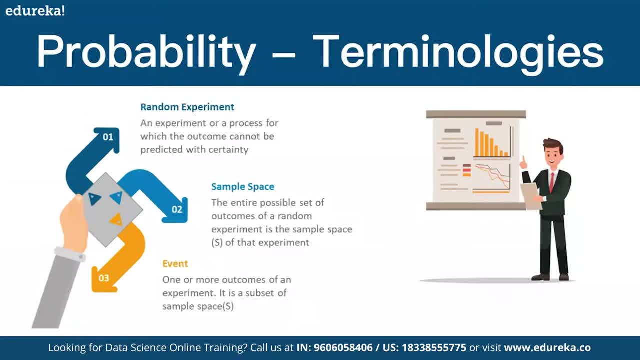 random experiment is an experiment where outcome cannot be predicted. so for example, on the highway there are accidents happening. let's say on the expressway or a highway. in a single day there might be zero accident. on the next day there can be 10 accidents. another day it can be one accident. so in the random experiment 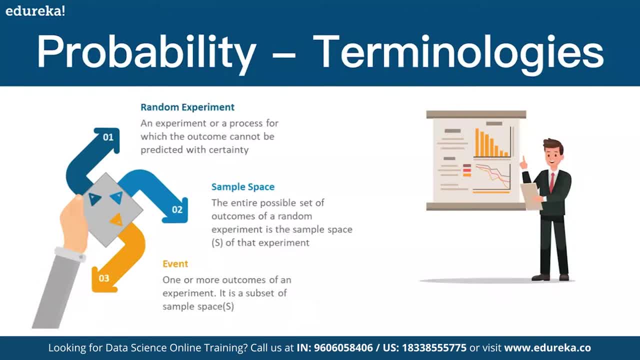 where outcome cannot be predicted. we cannot predict anything. what is going to be the future. that is called as a random experiment. sample space means the entire possible set of outcome of a random experiment. so once you perform a random experiment, you get different, different outcomes and that those different outcomes are known as a sample space. where all possible. 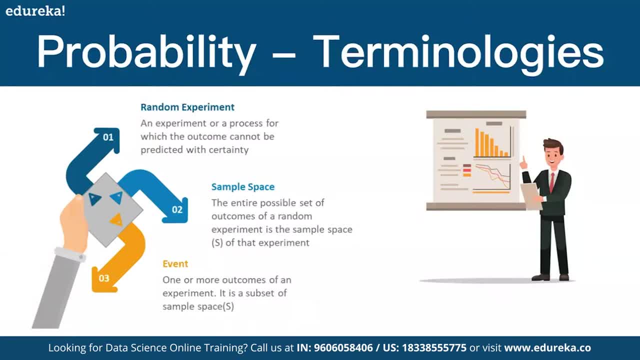 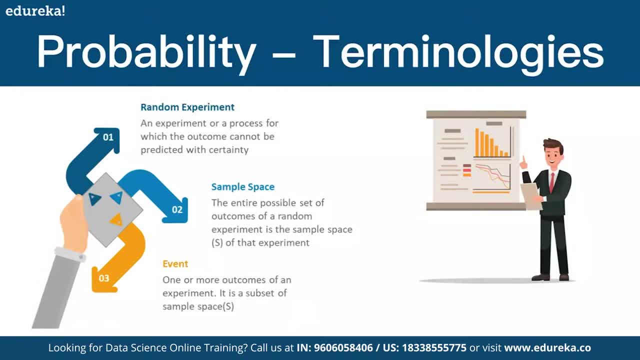 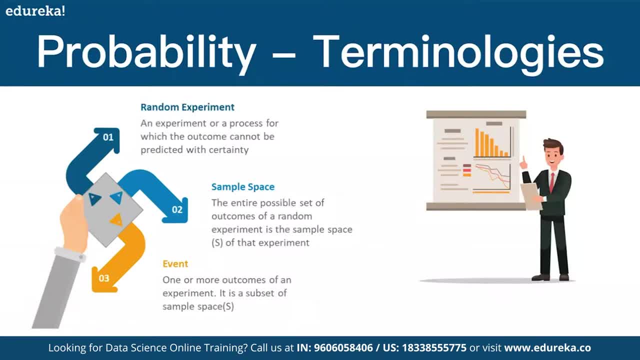 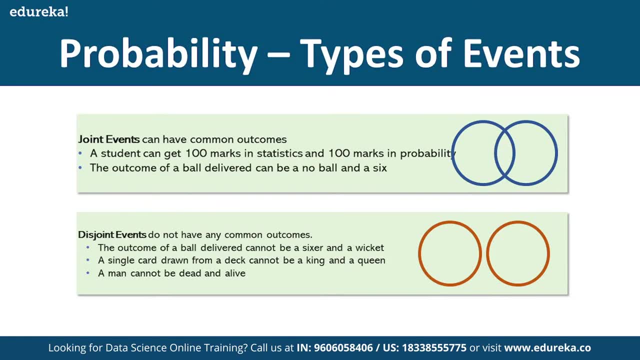 so let's say you perform experiment and someday you find three accidents, and someday you find two, two accidents, someday you find zero. so event is nothing but an outcome of an experiment. so these are terminologies we generally come across when we do machine learning. now, joint events happen by time. 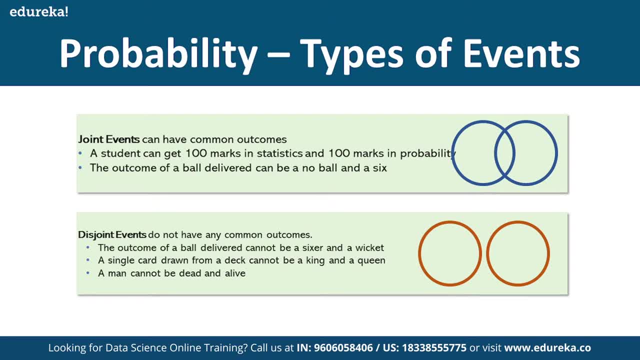 are what they have common outcomes. for example, a student can get 100 marks in stats and 100 marks in probability, so the same student is getting 100 marks in stats as well as maths. those are the joint events. the outcome of a ball delivered cannot be no ball and a six. so let's say a cricketer is. 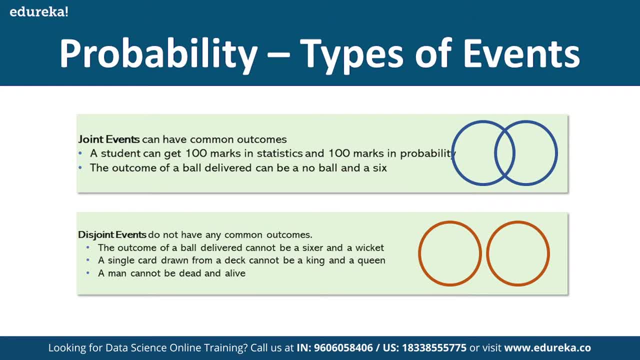 throwing a ball and the ball is no ball as well as six he is going to hit, so both are joint events. at the same time, on the same ball we got a six and we got a no ball. disjoint events are those which do not have a common outcomes. for example, outcome of a ball delivered cannot be sixer and 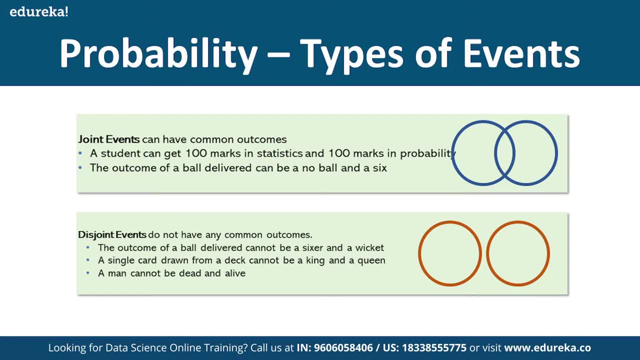 a wicket, so we cannot have a six and a wicket at the same point of time. a single card drawn from a deck cannot be king and a queen, so at the same point of time, king and queen cannot be there. it has to be king or a queen. these are called disjoint events. the man cannot be dead or alive. so at the 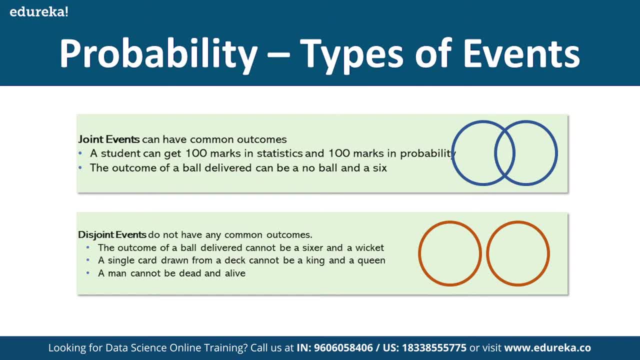 same point of time, the man cannot be dead or alive. so, at the same point of time, the man cannot be dead or alive. so, at the same point of time, the man cannot be dead or alive. either a man is dead or other man is alive. that is disjoint event, where there is no relation of one event with another. 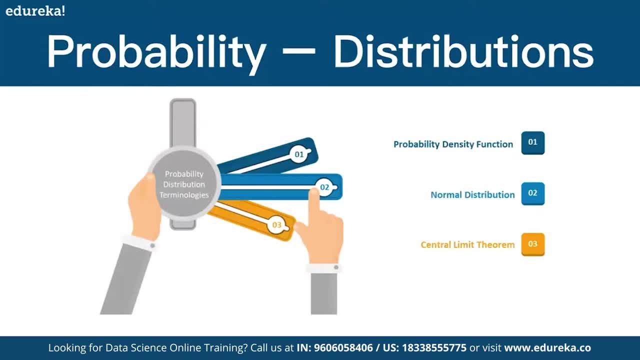 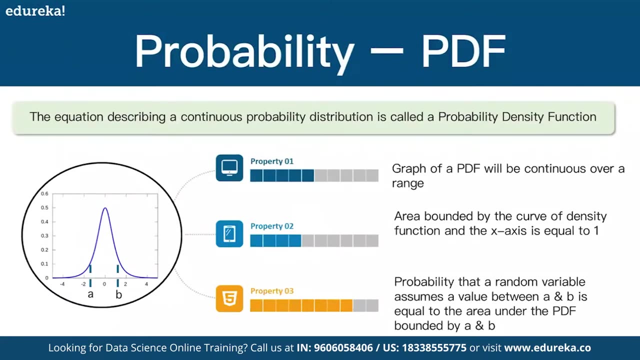 event. now there are three kind of probability distribution. one is called probability density function, another is called normal distribution, another is called center limit theorem. the probability distribution function means the equation describing a continuous probability distribution is called probability density function. so here we are, finding the density density means. 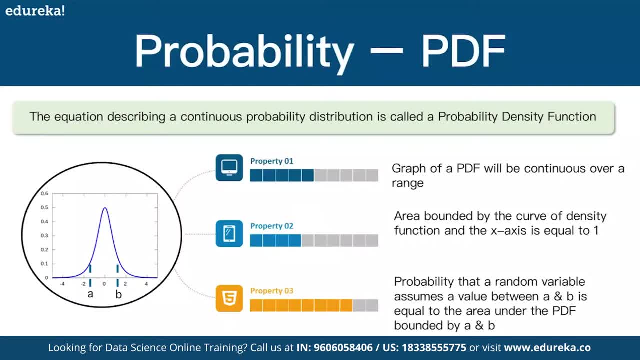 what event is occurring? maximum number of times and it is continuous in nature. so let's see, you are performing experiments continuously for 100 times and out of 100 times there are 60 times. you are getting the same kind of results nearby and you get one density. density means maximum. 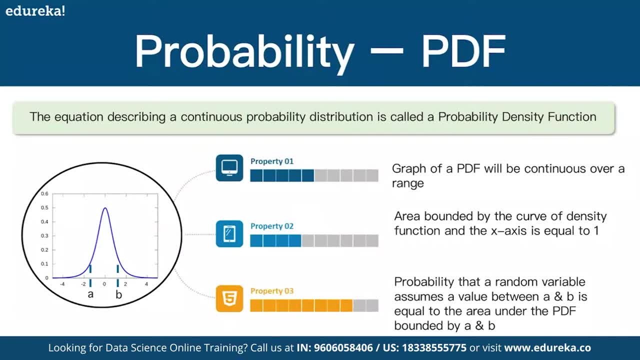 outcomes in the certain area that is known as a probability density function. so what are the properties of this graph? property of this graph is that graph of property distribution function will be continuous over a range, so let's say a range of the probability distribution function. So let's say a range of 0 to or minus 4 to 4, we are performing all the experiments and we get. 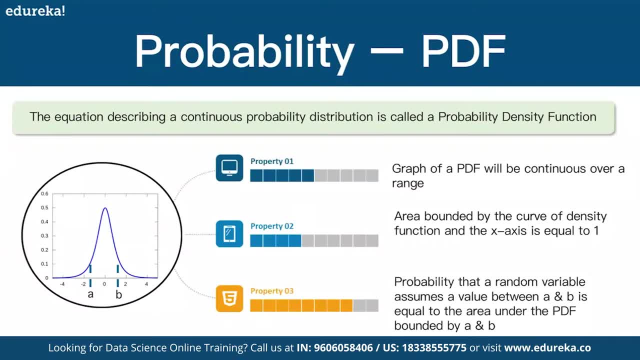 continuous distribution Area bounded by the curve of a density function and the x-axis is equal to 1.. So if you find the area of this curve with the x-axis, you'll find the area is 1.. Probability that the random variable assumes a value between a and b. 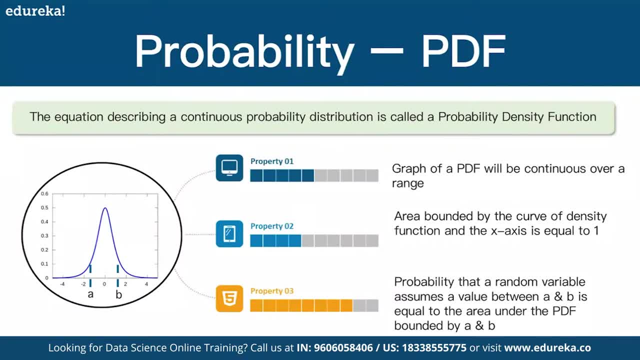 is equal to area under the probability distribution function bounded by a and b. So all the suppose you select any subset of the particular density function, you'll always find the answer is a subset of it. So answer is always between those two upper and lower limits. 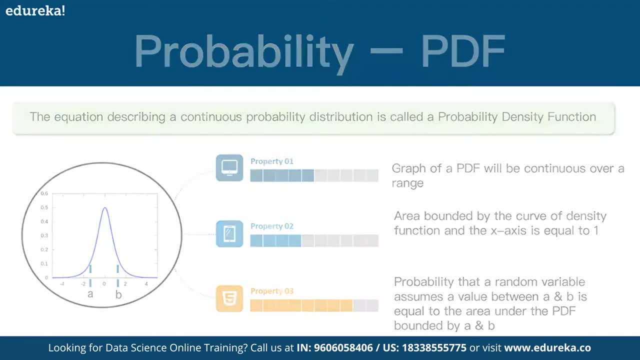 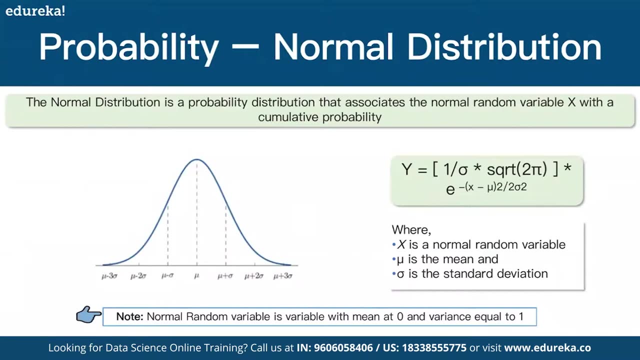 But that is known as the probability distribution function, density function. Now comes normal distribution, also known as the Gaussian distribution. Here, if you see the middle line, that's not as known as the Gaussian distribution. So that's the Gaussian distribution. 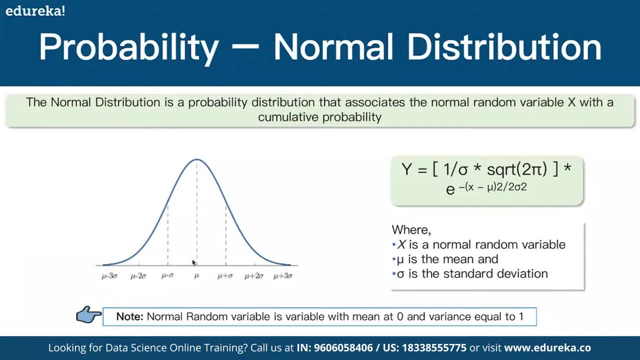 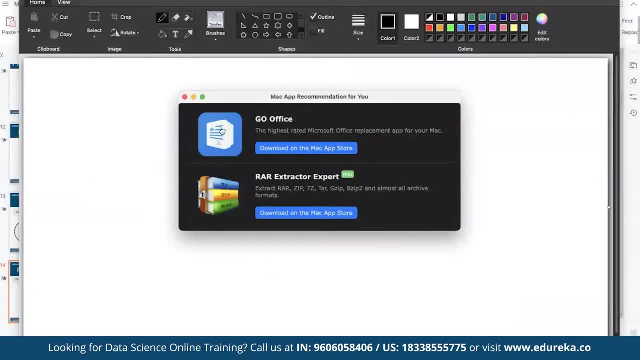 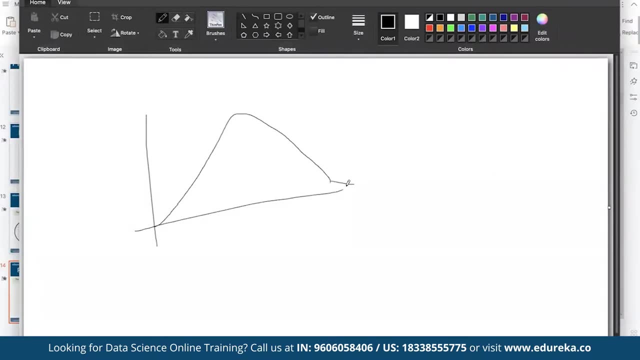 That's known as a mean value. So I'll tell you in the real time what is probability of normal distribution. So there's a scientist called Gauss who said that everything in this world is having a normal distribution curve. For example, this is a bell-shaped curve. You'll see very less people in the company, maybe three or four. 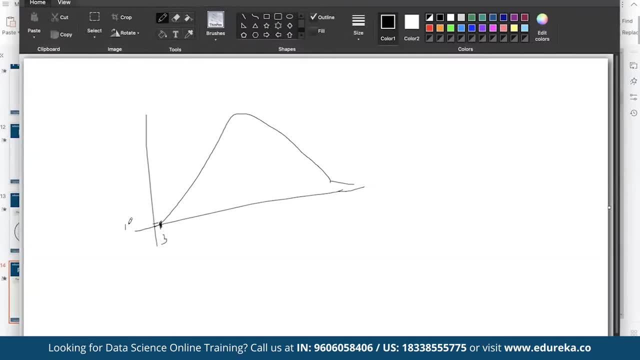 is having a very less salary, maybe one thousand rupees or five thousand rupees per month. This is salary And this is number of employees, And you'll see very less people in the company, maybe. so I will have to go the other way around, just let me. So this is number of people. 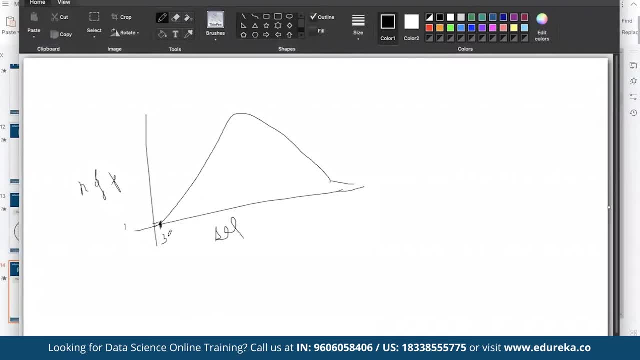 And this is salary. You'll see very less people are there in the company who have a salary, let's say, three thousand rupees per month, And this is number of employees, And this is salary, And this is number of employees. And this is number of employees And very less number of people. 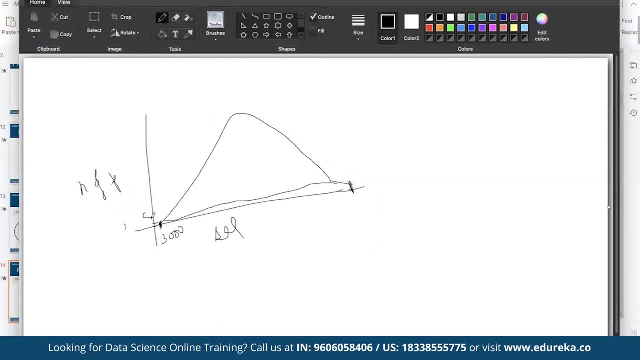 maybe four or five who are having a salary of more than five CR per month. directors of the company. Majority of the people lies in this area. You take any other example and it will fit into it. So Gauss said this is a normal distribution curve where majority of the people lies in the area. 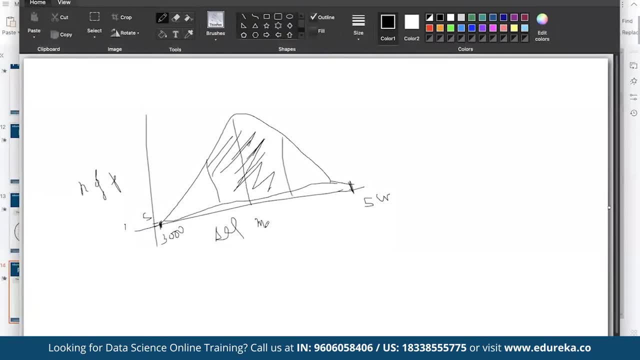 which is near to the mean value. So this is the mean value, And if you deviate from the mean, it is known as the standard deviation. So deviation from the mean is known as standard deviation. But this is what is explained in this graph. If you see the mean value, mu means mean. 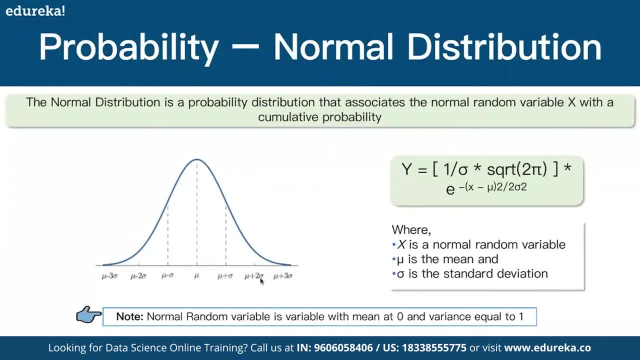 So here this is a mean value, mean plus one standard deviation, mean plus two standard deviation, mean plus the standard deviation. And this technique is also used for finding the outliers, And this technique is known as three standard deviation technique, three SD technique, where we find the standard deviation. 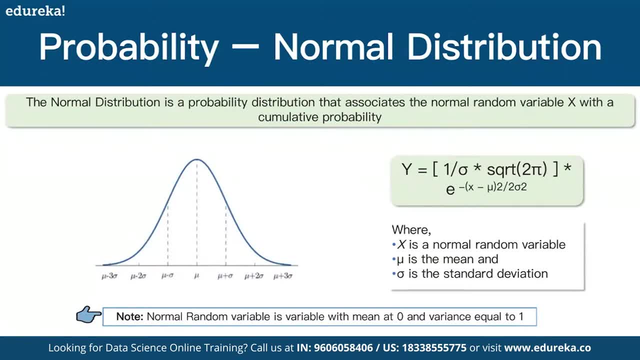 multiply by 3, add it to mean, that is upper limit, subtract from mean 3 standard deviation, that is the lower limit. So anything which is between the upper limit and lower limit, that is mu plus 3 standard deviation. 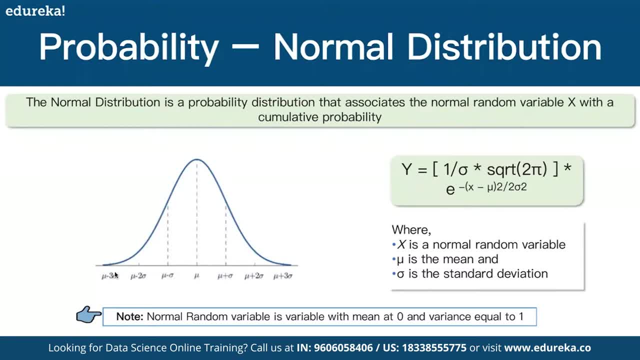 mu minus 3 standard deviation is called as a non-outlier. But anything which is coming out of this range lesser than mu minus 3 standard deviation, upper than mu minus plus 3 standard deviation, is called as an outlier. So this technique is generally used for finding the outliers in the data. 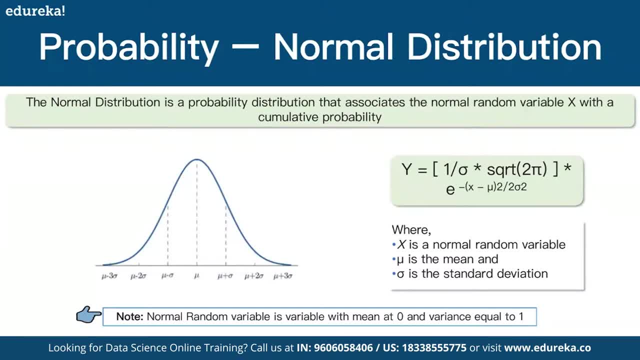 For example, you have an age column and all the ages are between 1 to 50 years And there is one value which is 1000 years. So no human being can live for 1000 years And that is an outlier. 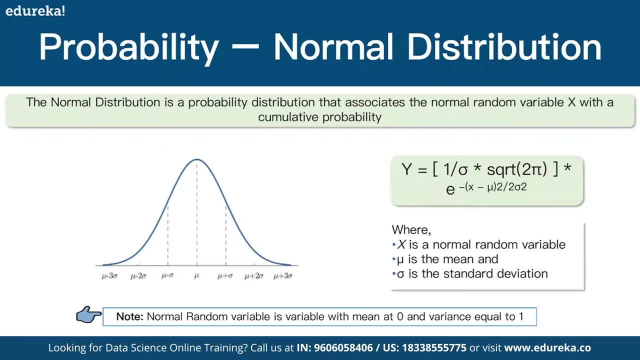 So we need to treat that outlier, We need to remove it or impute it or substitute it. So in the real-time data outliers can be there. So we need to find the outliers using 3 standard deviation technique. Other techniques are z-score. 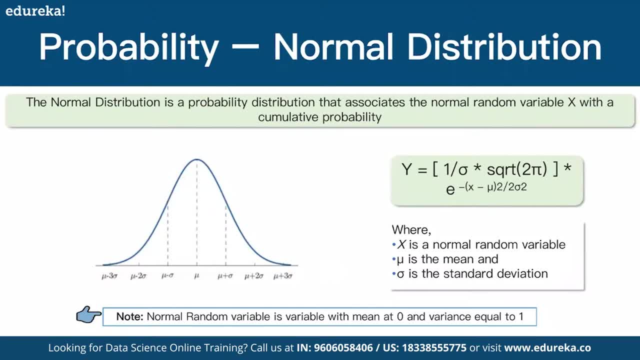 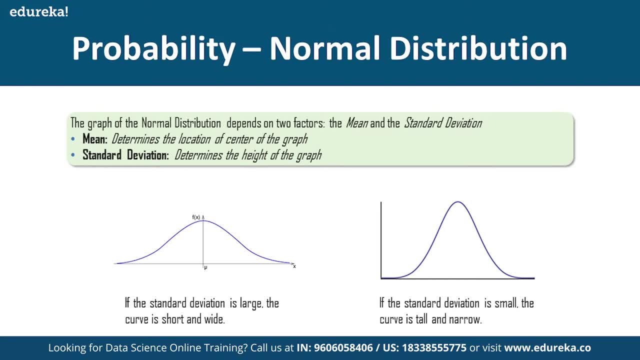 box-plot IQR method. there are different methods of it. The graph of a normal distribution depends on two factors: mean and standard deviation. Mean is the middle value. Standard deviation means how much you are deviated from the mean If the graph is having more height. 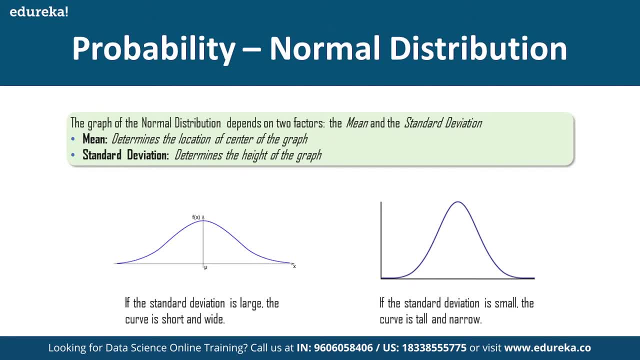 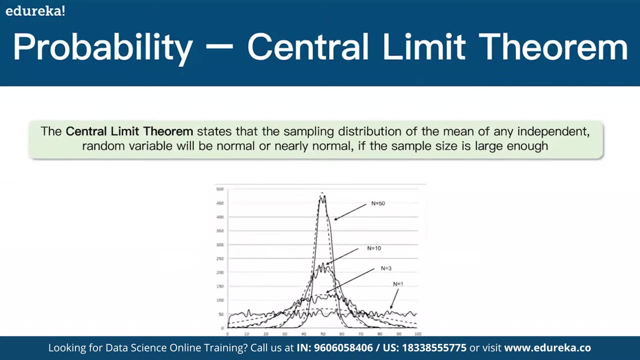 this bell-shaped curve is having more height, then it determines the standard deviation is nearby. But if the graph is something very much plateau, standard deviation is far away from the mean. The central limit theorem states that sampling distribution of the mean of an independent random variables will be normal or nearly normal. 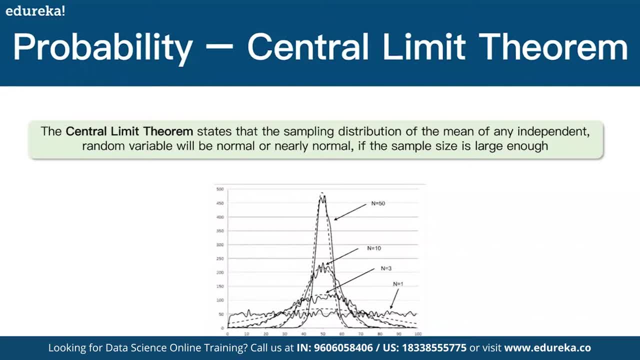 So let's say you have a population of 1000 records, or you can say 1000 experiments and if you plot it you will find most of them are lying in the normal distribution curve. So maybe this is one experiment. second experiment, third experiment: 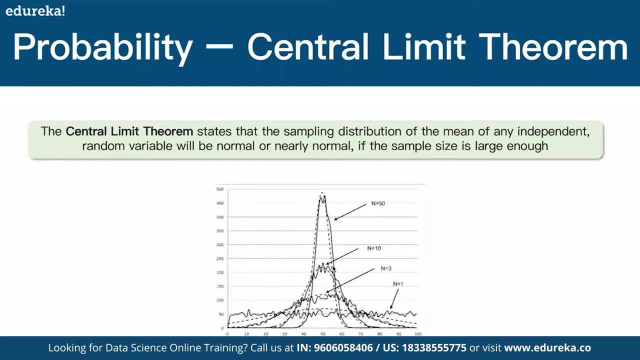 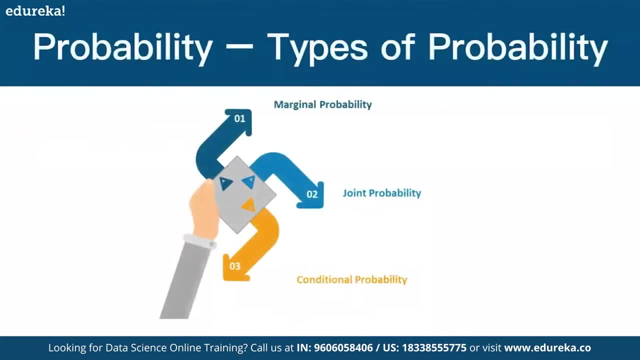 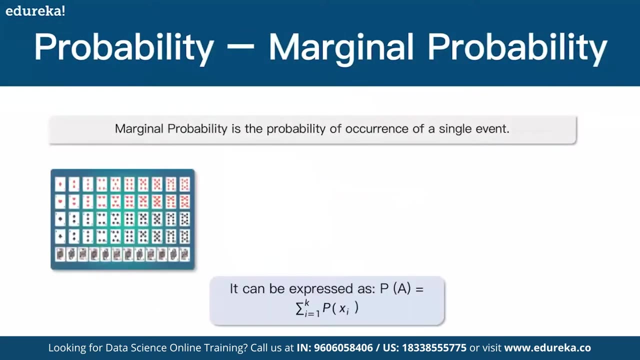 fourth experiment and so on, But they are always following a normal distribution curve That is known as the central limit theorem. Now there are three types of probabilities: marginal, joint and conditional. So this we have already read in 10th standard. 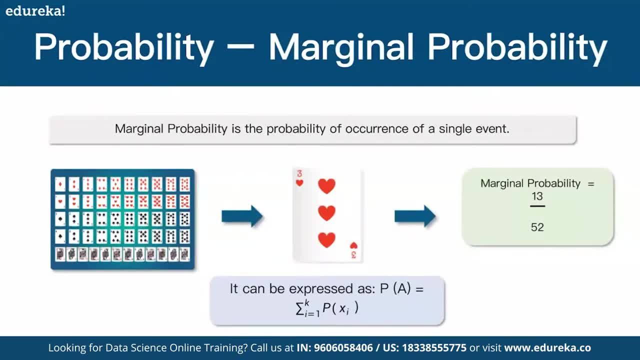 Marginal probability is a probability of outcome of a single event. Suppose I want to find all spades, all hearts, all diamonds. So there are total, how many hearts in the in the deck of cards- 13.. So what is the probability of getting a heart-shaped card? is 13 by 52.. 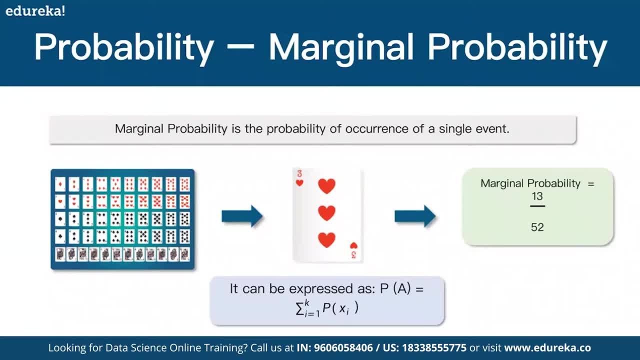 Probability of a single event. So I want to find the probability of an event that I get a heart-shaped card. Let it be any number. If my question is: I want to find out heart-shaped card, let it be any number. So total 13: heart-shaped card is there. 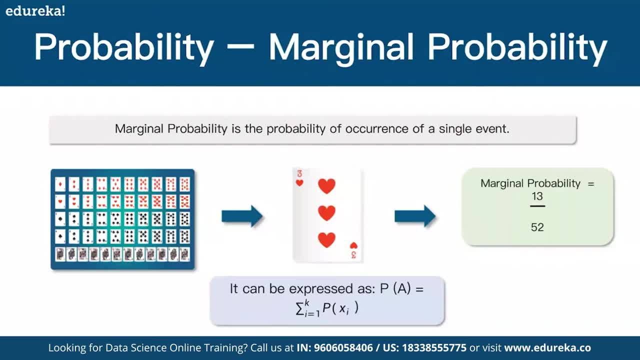 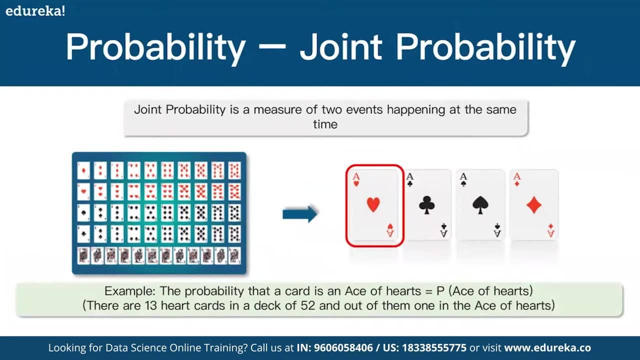 Heart. 13 by 52 is the total number of cards. We get the probability That is known as the marginal probability of outcome of a single event. Marginal probability means probability of a single event to occur. Then comes joint probability. Suppose I want one more condition, that I want heart-shaped ace. 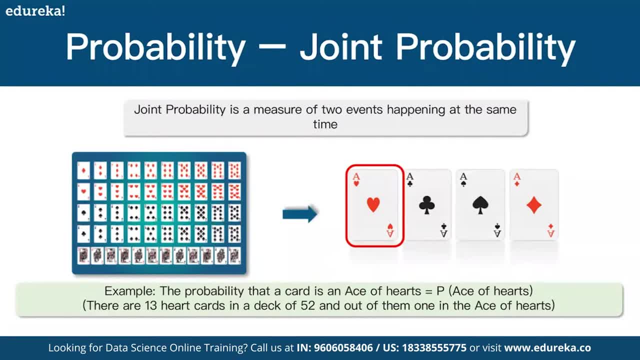 So there are two conditions: Heart-shaped. Another condition is ace, So the probability that a card is ace of heart. So there are 13 heart cards in the deck of 15.. Out of them, one is ace of hearts. That is known as the joint probability. 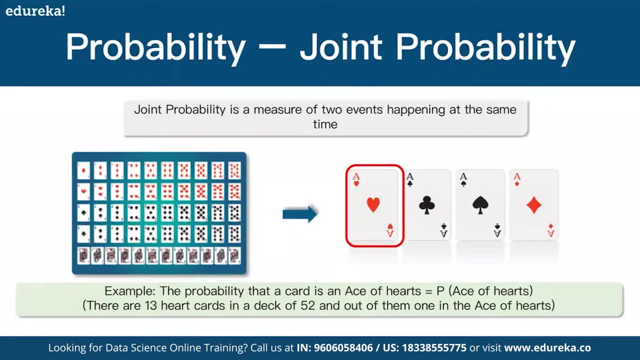 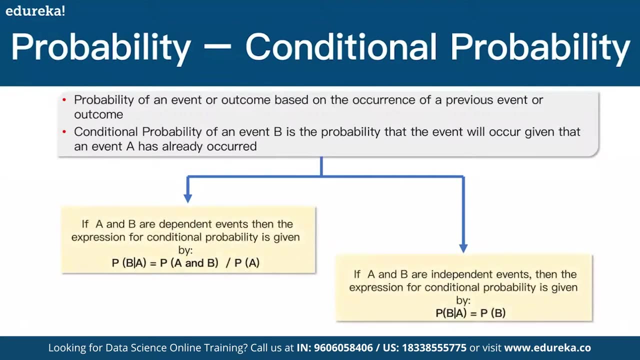 Probability of one event, Along with the probability of outcome of that event again. So first I pick up the heart-shaped card. Within those heart-shaped card, what is the probability of picking ace? Conditional probability means probability of an event which is dependent on another event. 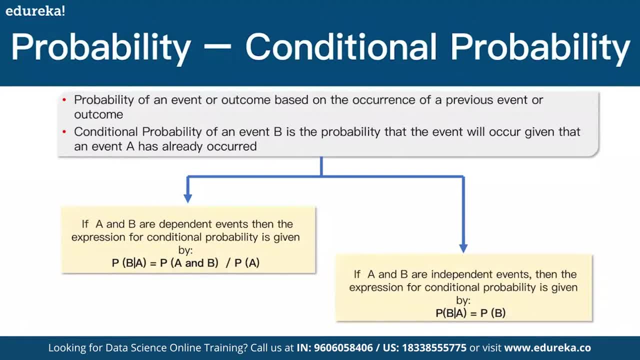 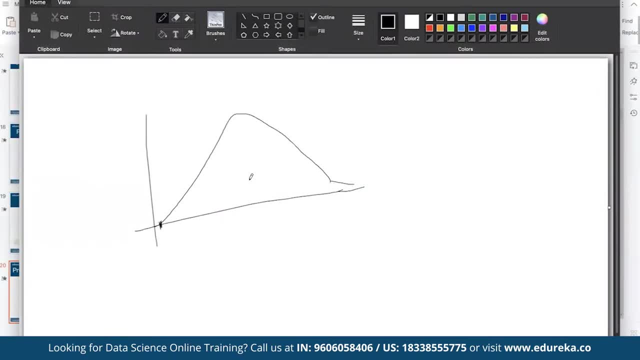 So here it reads: P A by B. So how do we read this? Let me explain you. Conditional probability is given by Gauss again, And also known as naive-based classifier. In machine learning it is also known as naive-based classifier. So what is the formula of naive-based classifier? 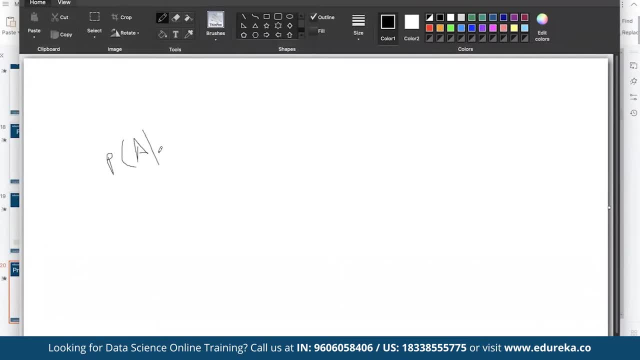 P A by B is equal to P A, P B by A. P A by B is equal to P A. P B by A. Now how do we read this This? A is known as unknown, B is known as known. What is the probability of event A, given that B happens? 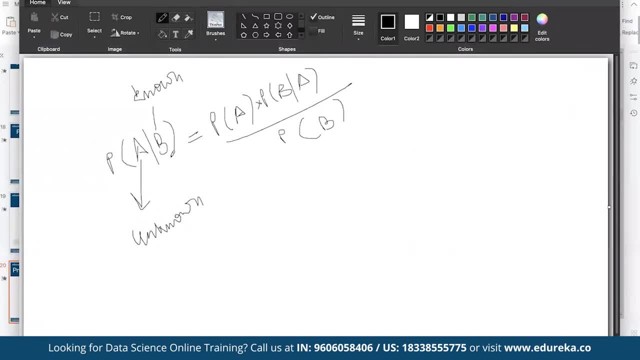 So how do we read? What is the probability of event A, given that B happened in the past? For example, what is the probability of dengue fever if the person fever is 104 degrees? What is the probability of lung cancer if the person is smoking 10 cigarettes a day? 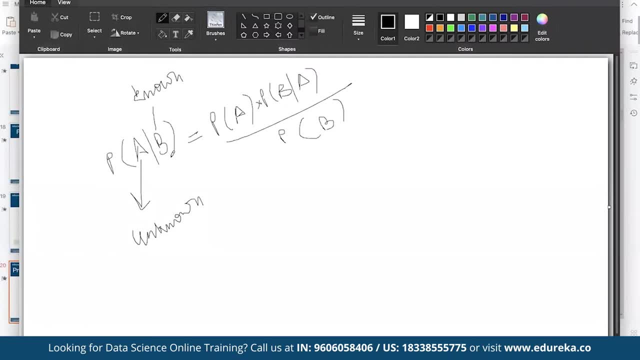 What is the probability of rain if we see the clouds? So this is known as a conditional probability, where probability of one event depends on occurrence of another event. Right? So what is the probability of passing an examination if the student studies for 10 hours a day? 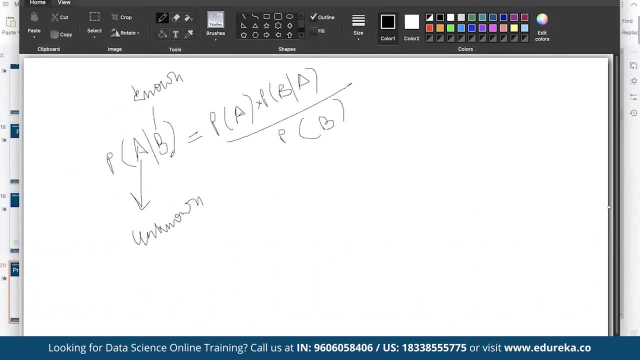 So all the conditional probability problems generally used in bioinformatics or medical domains are getting the answers for the disease, for the new launch of a drug. Let's say there is a new launch of a drug for treating, let's say, dengue fever. 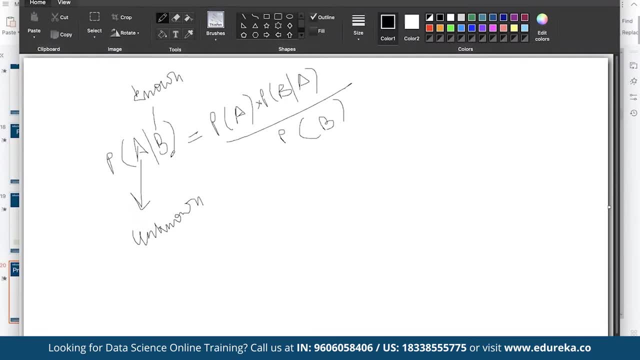 We use conditional probability that if we give a dose of 5 mg, the probability of fever getting over in 3 days is 90%. If I give a dose of 15 mg, the probability of fever going in 2 days is maybe 90%. 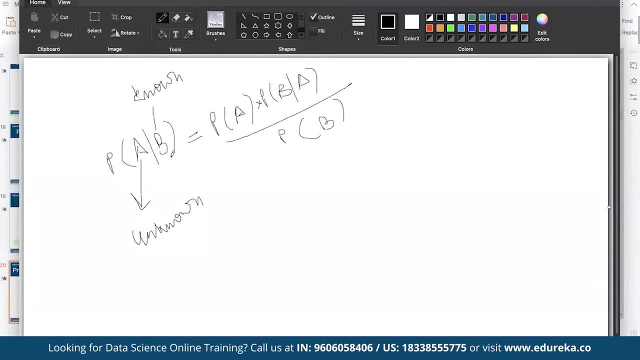 Conditional probability is used when we have probability of a known event and we want to find the probability of an unknown event Right. And this machine learning terminology, this algorithm, is known as Gaussian NB- Gaussian NB- Naive Bayes. So conditional probability is probability of an event outcome based on the occurrence of 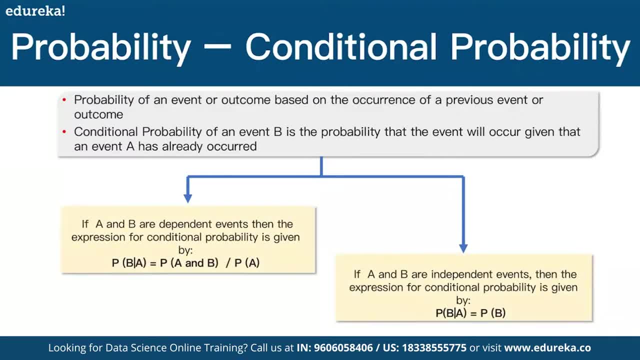 previous event or outcome. So when anything happened, what is the outcome of next event? We call it as conditional probability. Conditional probability of an event B is the probability that the event will occur, given that event A has already occurred. If some event has already occurred in the past, 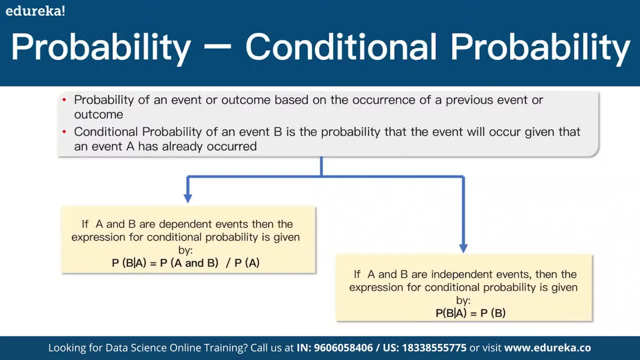 what is the probability that the next event will occur after that event? If A and B are independent events, then the expression of conditional probability is given as P B by A equal to P B. So generally conditional probability is used when the events are related to each other. 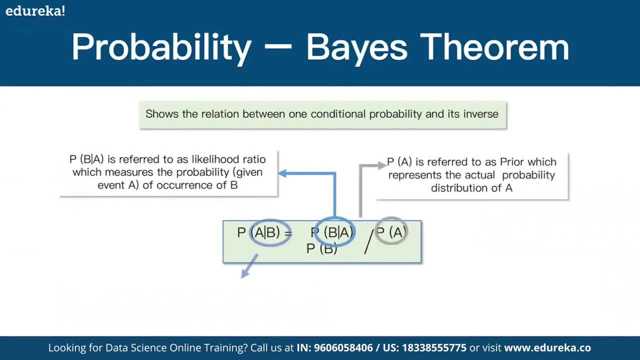 So this is Bayes theorem which I discussed with you: P A by B equal to P B by A into P B divided by P A. P B by A is referred as likelihood of ratio, which measures the probability of given event A for the outcome of B. 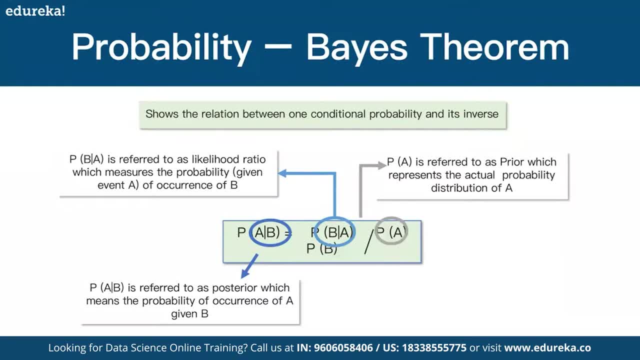 So here P, B by A means what is the probability of B given that A happens? And here what we need to find: what is the probability of event A given that B happens? Now probability of the Bayes theorem can be used to find out problems. 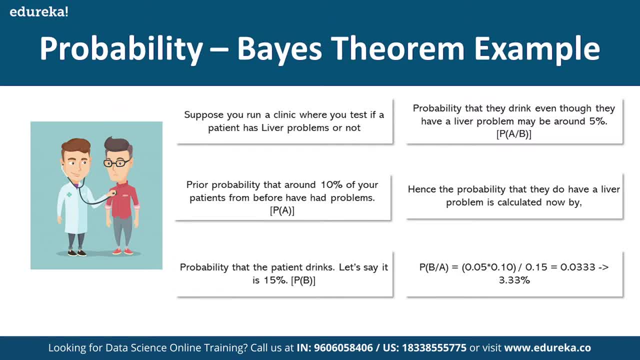 Like: suppose you run a clinic where you test if the patient has a liver problem or not. Suppose you are having a clinic and liver patient comes there. Probability that the person drink has a liver problem is 5%. Probability that 10% of your patients from before have had problems. 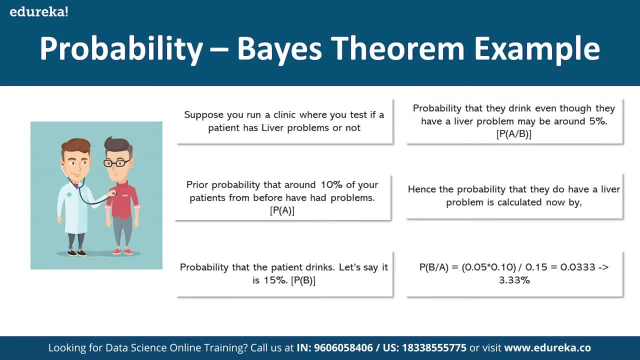 So all the patients which you have seen till now, 10% were having liver problems. Hence the probability that they do to have a liver problem is caused by now. And what is the probability of liver disease if the patient drinks is 15%. 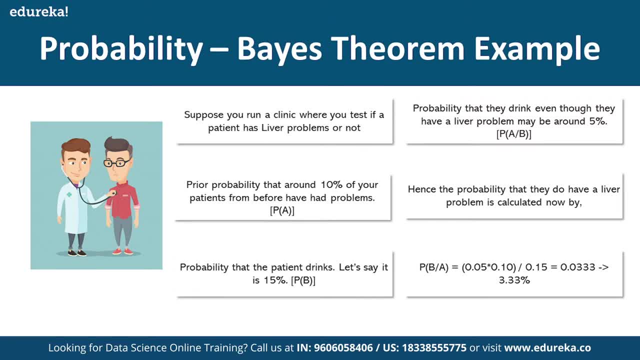 So we will find P B by A. That is probability of liver disease if the person drinks on the everyday. So this is just a small example where we are discussing about what is the probability of one event, provided another event happened in the past. Now, if we talk about applications of probability, 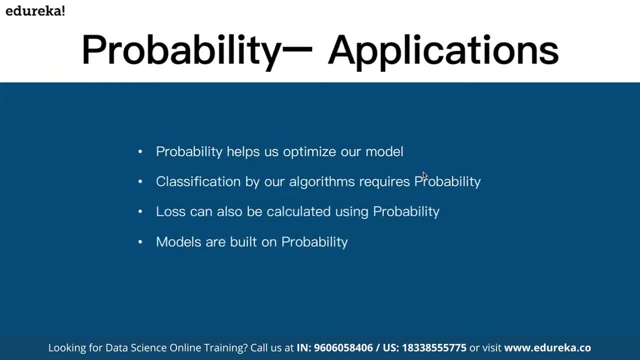 probability helps us to optimize our model. Optimize means it helps us to take a better decisions. For example, if you run a linear regression algorithm, your data should be normally distributed. If your data is not normally distributed, you cannot expect good results from linear regression. 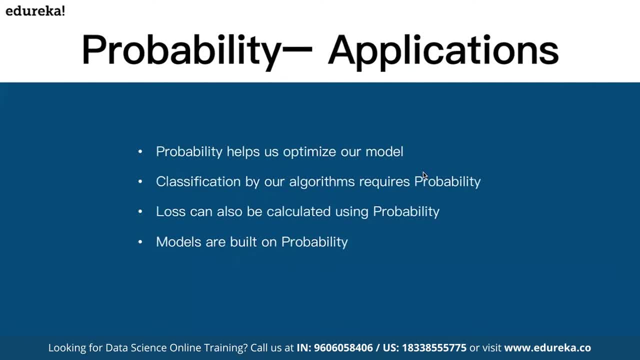 Classification by algorithms requires probability. So when you are talking about logistic regression, logistic regression requires probability values of an event. In those cases, probability plays a very important role, because logistic regression is all about probability of an event: whether it can happen or it cannot happen. 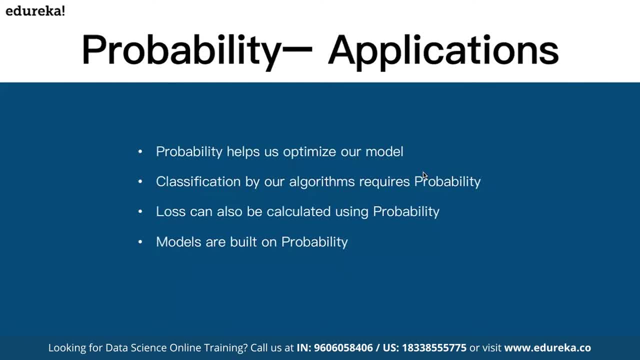 If the probability is above 0.5, we say it will happen. If it is below 0.5, we will say it will not happen. So all the classification algorithm, so whenever you see in machine learning classification world, all the classification algorithms belongs to. 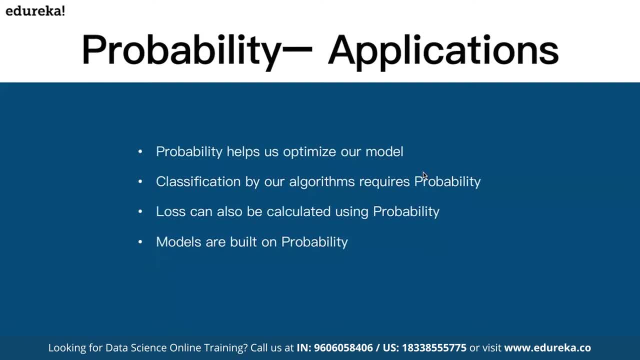 probability problems. So all the classification problems means whether the hotel is 2 star, 3 star, 4 star or not, or whether this event will occur or not occur, whether a person will fail in the class or pass in the class. 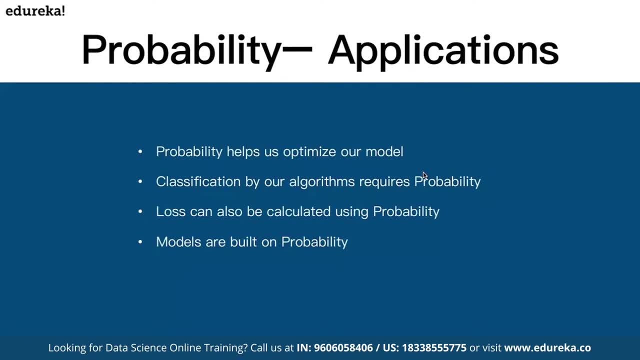 All the yes or no, true and false, maybe 3 or 4, 5 categories will work. So all the probability problems use classification problems. Loss can be calculated using probability. Models are built on probability. So majorly all the machine learning algorithms. 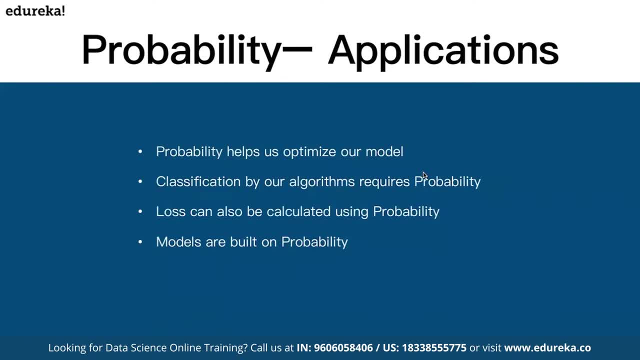 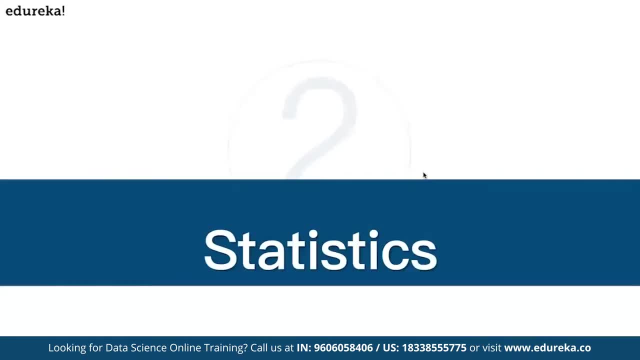 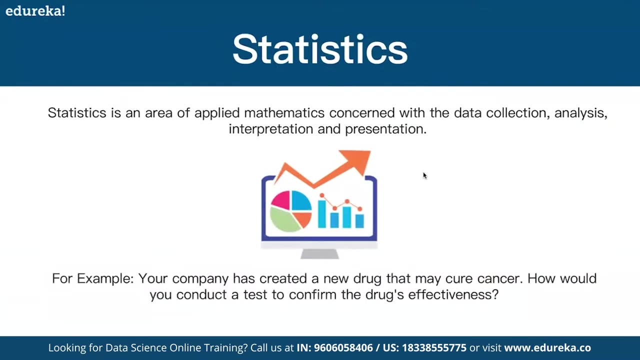 are using probability values at some point or the other, maybe at the time of finding the accuracy, or maybe at the time of finalizing things. Now, what is statistics? Stats is the area of applied mathematics concerned with data collection, analysis, interpretation and presentation. 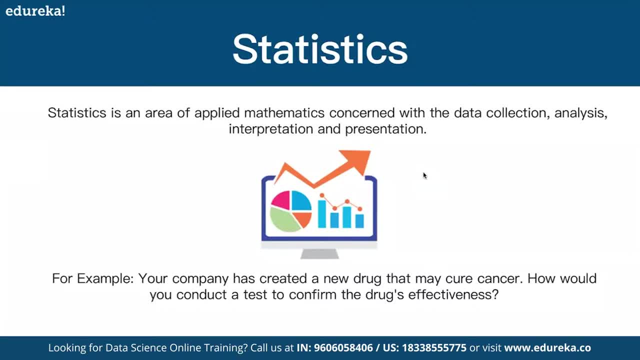 So what is stats all about? Stats is all about applying mathematics, which is primarily dealing with collecting data from different sources, also known as data mining, analyzing it to the next level. whether the outlier is there or not, correlation is there or not. 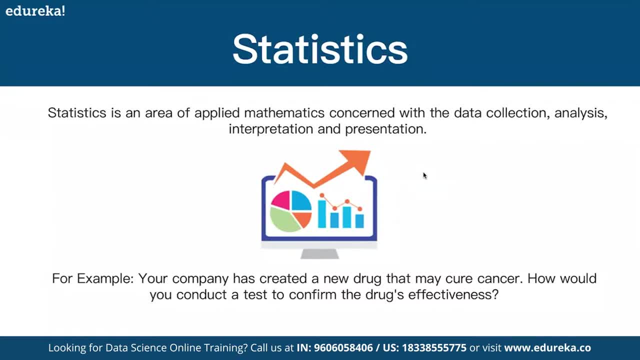 skewness in the data is there or not, normally distributed or not, interpret it, digest it, ingest it and present it. That is the purpose of stats. So the sole purpose of stats is to find the hidden insights in the data. 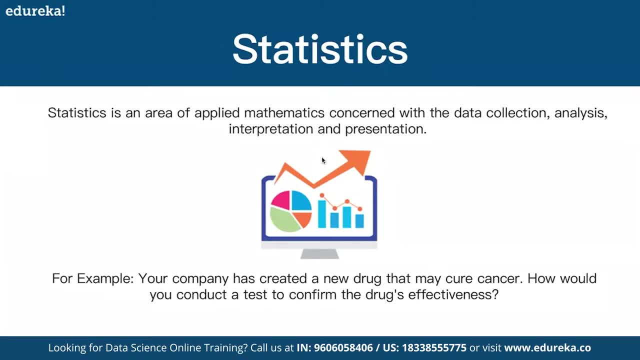 For example, your company has created a new drug that may cure cancer. How do you test to confirm the drug effectiveness? So there are multiple types of tests in statistics which confirms that this drug is going to work well, So stats is used to figure it out. 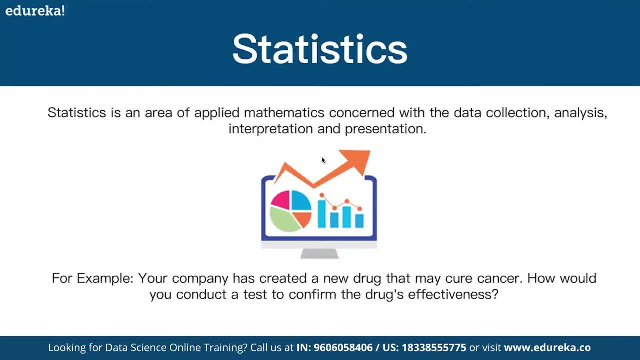 what happens on the population or a sample and based on that we take some predictions and confirm that this thing is surely going to happen. So stats is a backbone of machine learning. So I told you, machine learning is all about predictive analytics, When you want to predict future based on historical data. 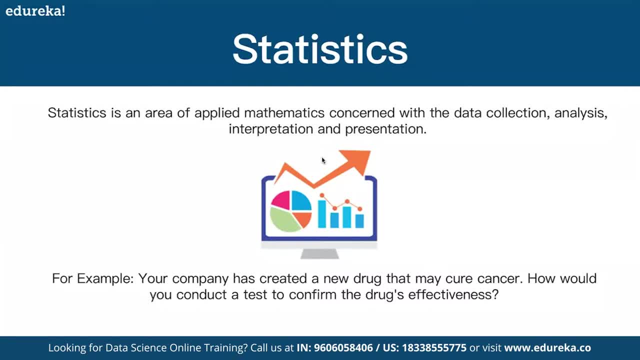 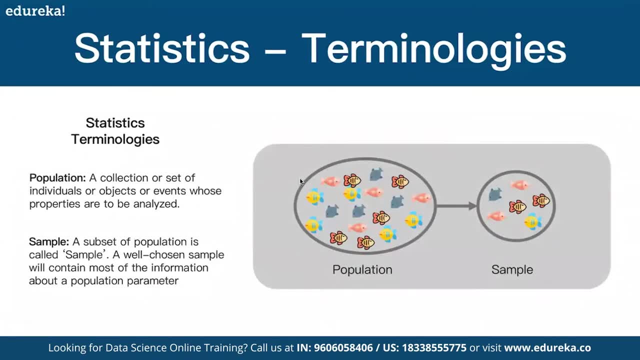 we say we are doing machine learning, So stats is a backbone of it. If we talk about statistics, terminologies, we have a terminological population. Population means everything and anything: Collection or a set of individual or objects or events whose properties are to be analyzed. 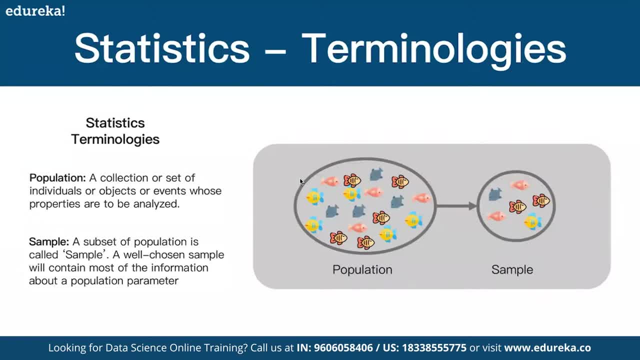 Let's say I give you Amazon whole data. Last one year data from Amazon I have given you and you see all the age group people are shopping, Maybe a 15 year old boy to 70 years old person, buying different things based on different age groups. 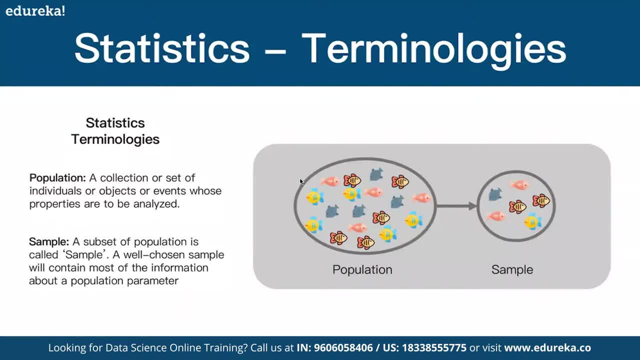 different professions, different likelihood, different geographical areas, And if I've given you everything and anything with my database to analyze and that's known as a complete population Sample, is what? Sample is a subset of population Which is chosen based on the some parameters. 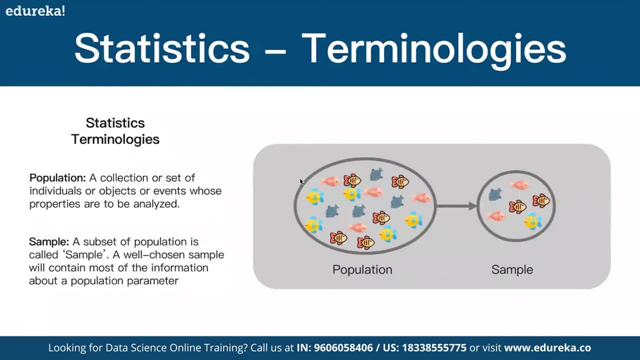 Suppose I want only people within the age group of 15 to 20 years of last two years What they have bought. Suppose Amazon wants to analyze between the 15 to 20 years of age group Generally, these students or these kids or teenagers. 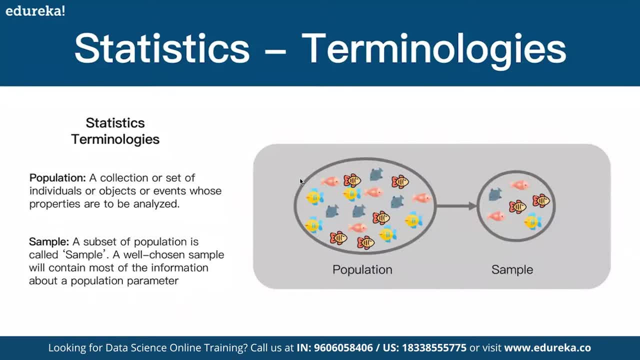 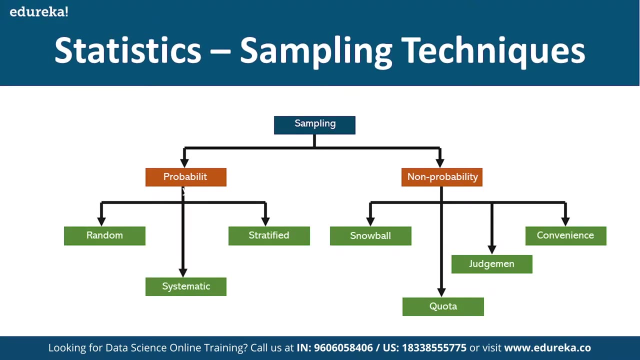 they like, what They most of the time buy what And based on what they want to promote sales. And that is a sample from the huge subset, huge, huge data set. We are picking up things as per our interest, So there are different sampling techniques. 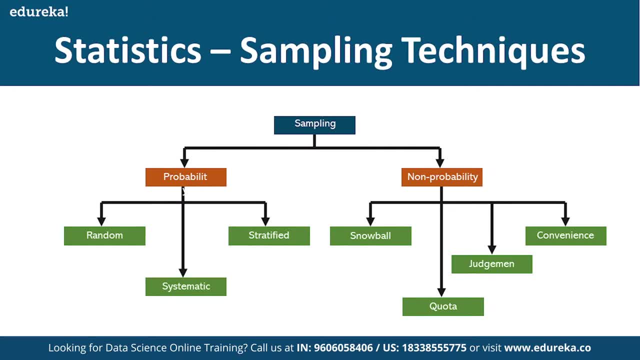 So one is probability, Another is non-probability. So in probability we will take some random data or systematic or stratified, And non-probability ways we take snowball, quota, judgmental and convenience. So there are different ways of sampling depending on 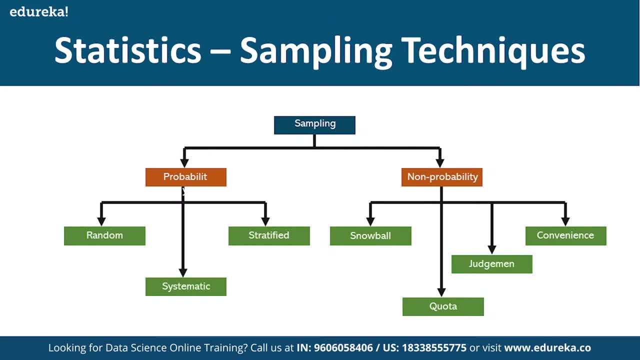 whether we want to go by probability of event to happen or not, Or whether we are not worried about the probability of an event. We will not go deep into all this. They itself is a big story altogether. Different techniques, Now. there are three types of sampling. 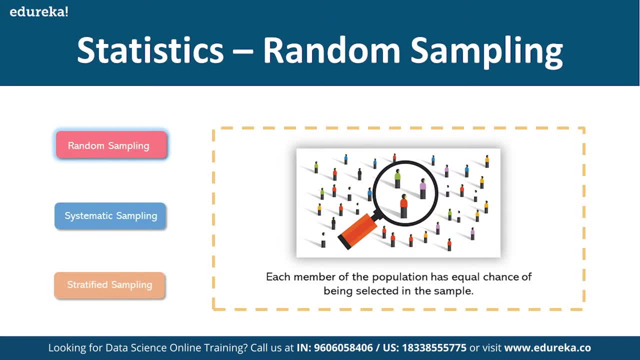 One is random sampling. Random sampling means each member of population has an equal chance of being selected in sample. Like lucky draw. What is lucky draw? Lucky draw means suppose everyone buys some ticket for lucky draw. We put it in a big container. 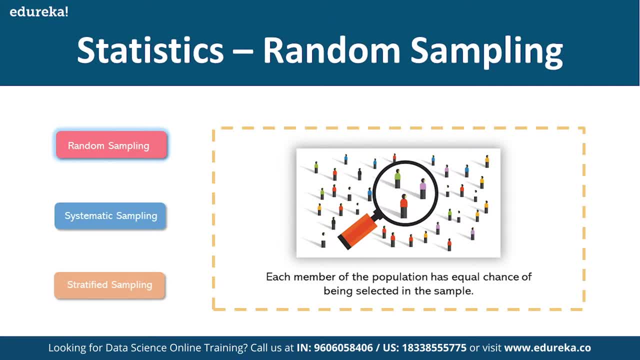 And somebody picks up only one chit, And that person is a winner. So every member has a likelihood. Like KBC, you might have seen on the television On Banya Karupati. What is there? Millions of people are answering the questions. answer. 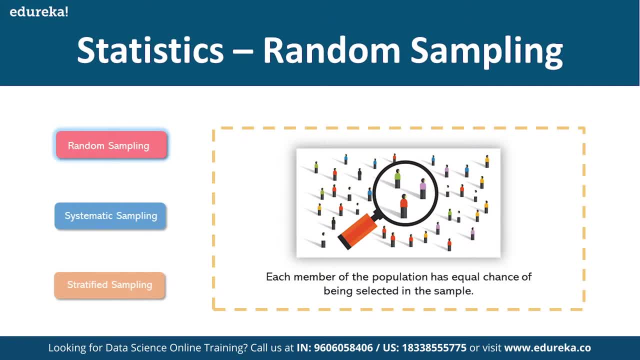 And system is randomly picking one of them who have given the right answer, And each member who is giving the answer for KBC has a chance to win. And that is known as a random sampling- Picking up a sample from the whole population. 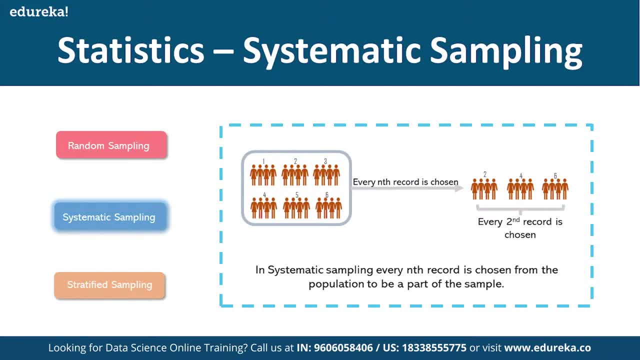 Another is systematic sampling. Systematic sampling means sampling every nth record from the population to be part of sample. So let's say I make students of a class stand in a queue And I will pick the third student from every queue. So let's say I ask students to 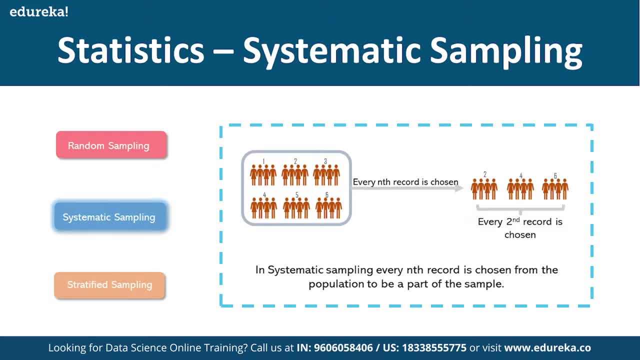 stand up in a group of four. So there are four groups, Maybe five groups are there, Or six groups are there, And out of all these six groups I picked up only the third person from that group, So that is known as stratified. 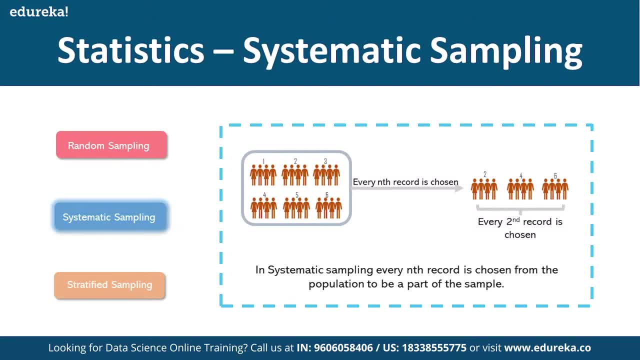 Stratified means the particular record has been chosen from every sample So that real-time example can be. you are choosing from every state of India. you are choosing one person who is a topper of mathematics from a particular state. So you are choosing one topper. 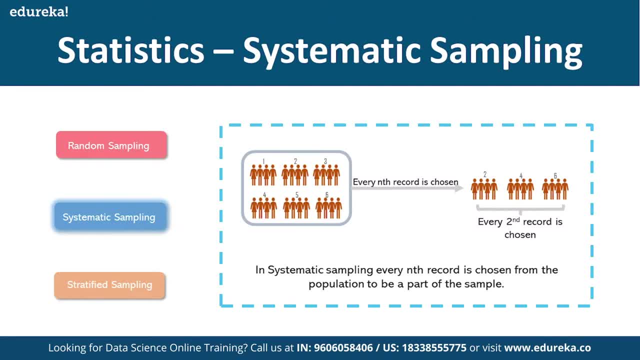 from mathematics, from every state, And you are getting 26 toppers And those are called as a systematic sampling. You are based on some criteria, Based on some numbers, Based on some preference. You are picking up a particular record from a sample. 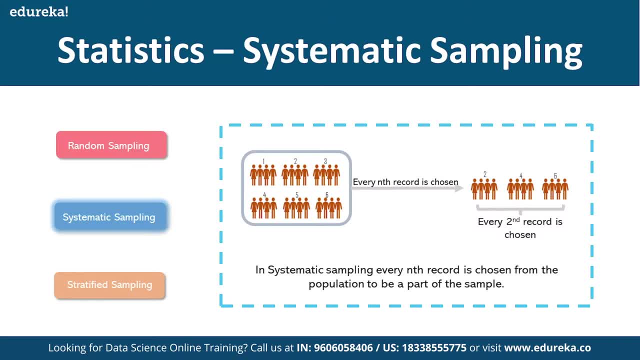 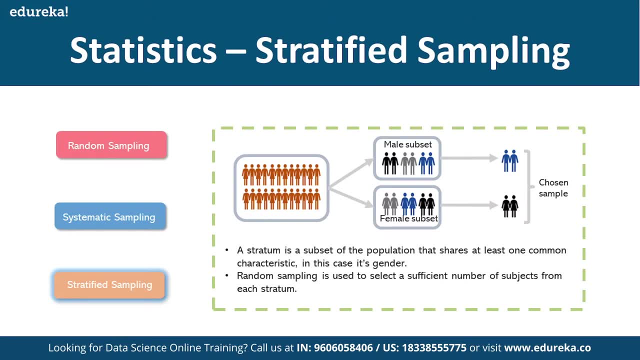 And that is known as stratified. Like nth record is chosen from here. Stratified means stratum. Stratum means a subset of population that shares at least one common characteristic. For example, in a class you ask all male students to stand together or all females to stand together. 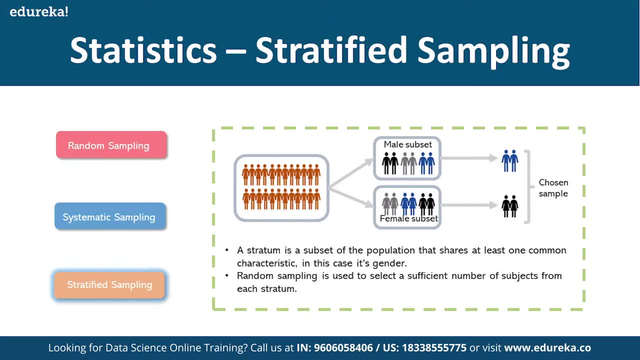 And then you are choosing from the male sum samples and from female sum samples. So that is known as a stratum or stratified sampling. So random sampling is used to select a sufficient number of subjects from a stratum And once you are doing stratified, 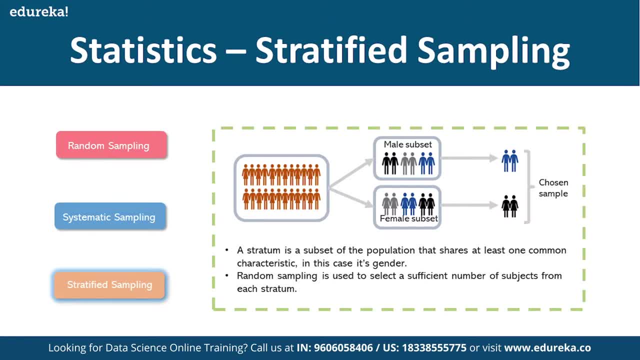 stratified means selecting everything which are same. You are picking randomly from there. That is known as stratified random sampling. So these are different sampling techniques And generally used in all the bioinformatics checking the soil type. So you are collecting a soil of a particular state. 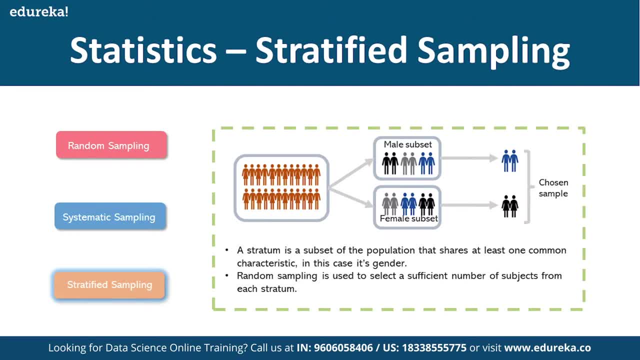 after every 20 kilometers to take a sample of a soil And you sow some seed into all the types of soils And see which plant is growing fastest and which plant is the most healthiest one. So that is called as a sampling technique, where you pick up some sample. 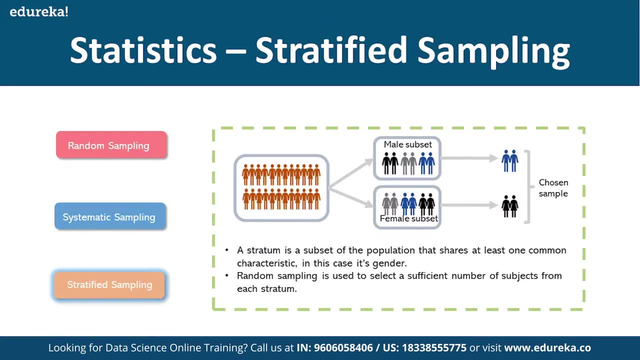 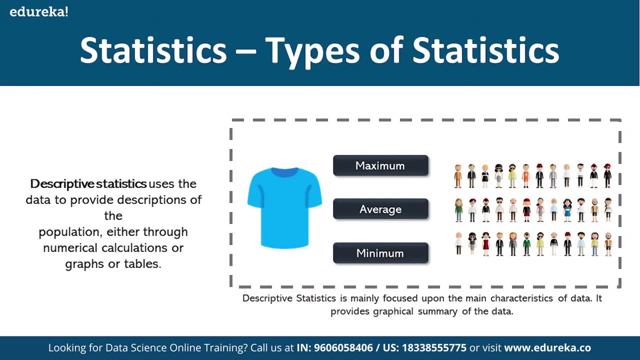 and check how the whole population is going to behave. Now, there are types of statistics, if you talk. There are descriptive statistics. Descriptive means maximum, average and minimum It describes who is going to be the maximum in weight, Who is going to be the average in weight. 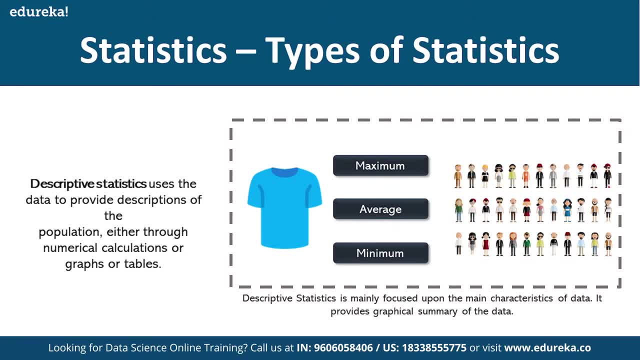 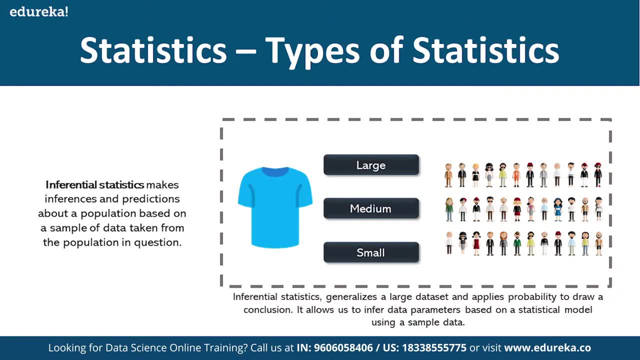 Who is going to be the minimum in the weight. That describes. So maximum, minimum and average are the descriptive statistics matrices. Similarly there is called inferential statistics where we have large, medium and small. This is comparative. That is known as a 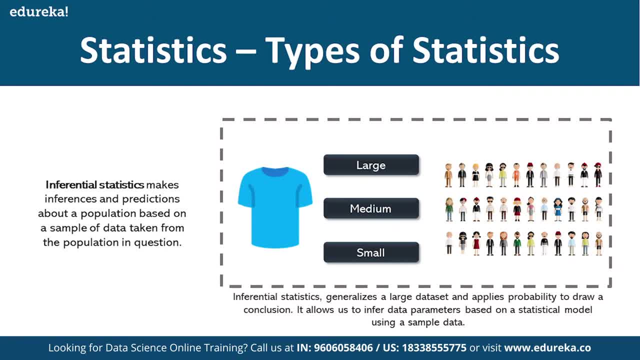 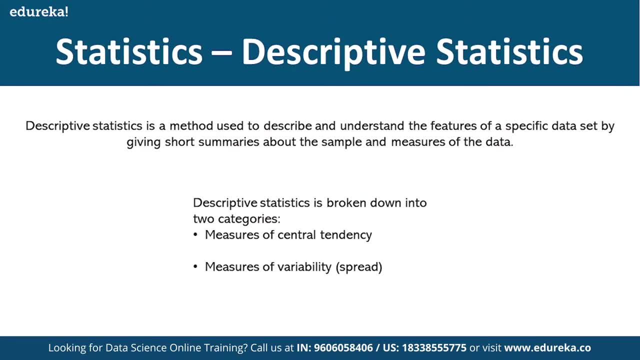 inferential statistics We find the inference. So inferential statistics makes inference and predictions of population based on sample from the population of the portion. Now, if you talk about descriptive statistics, descriptive statistics is used to describe the features of a given subset and it measures. 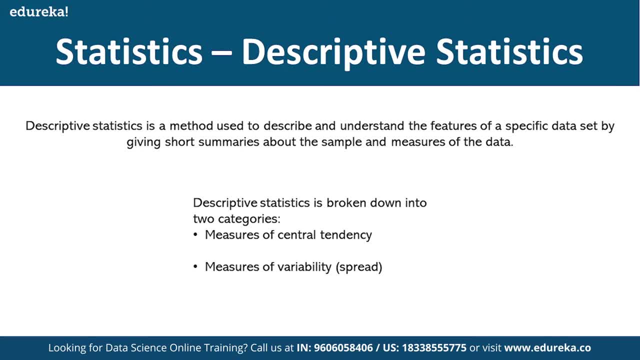 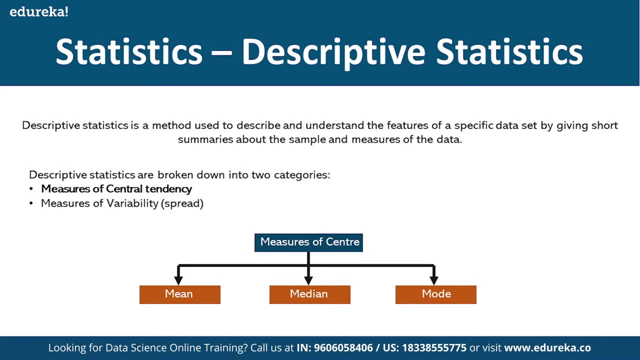 It is broken down into measure of central tendency and variability. Descriptive statistics is again of two parts: Measure of central tendency, measure of variability. That is how differ from each other. Descriptive statistics for central tendency means mean median mode. 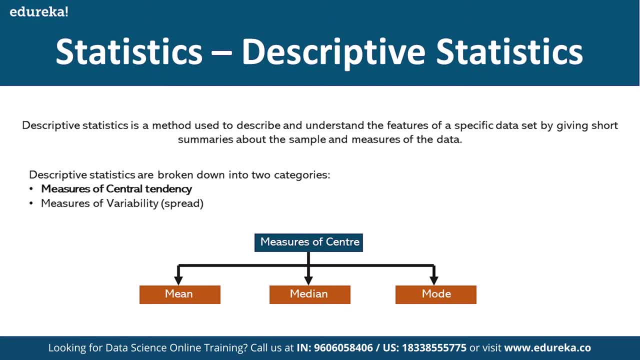 What is average? What is the maximum occurring value? That is mode. What is the median? What is the middle value? Mean, median mode is very common, Commonly used term and you might have got it in 10th standard also. So mean is average. 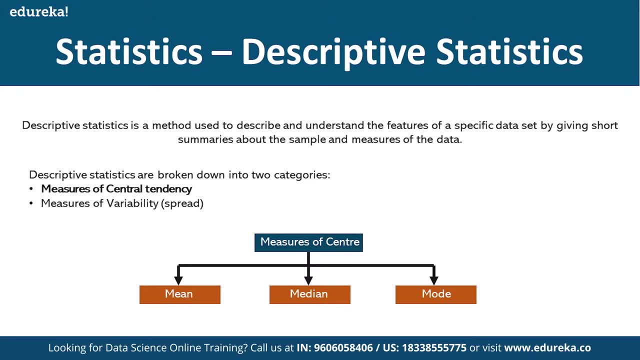 of everything, Median is middle value. If you sort data in ascending order and find the middle value, that is, median Mode is a maximum occurring value. Range is nothing but range of values between 10 to 100, 100 to 200.. That is range. 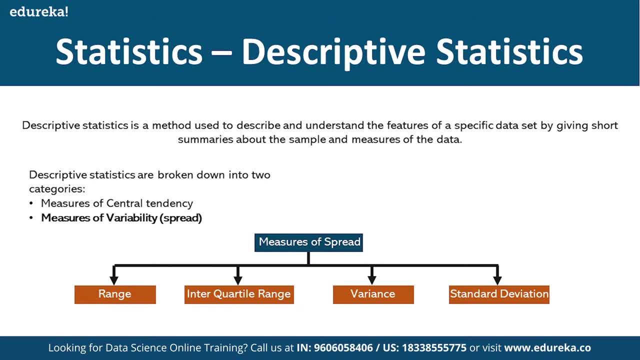 Quartile means first quartile, second quartile, third quartile. You might have heard about percentile. Percentile is a comparative study, So quartile means first 25%. second quartile means 50%. third quartile means 75%. 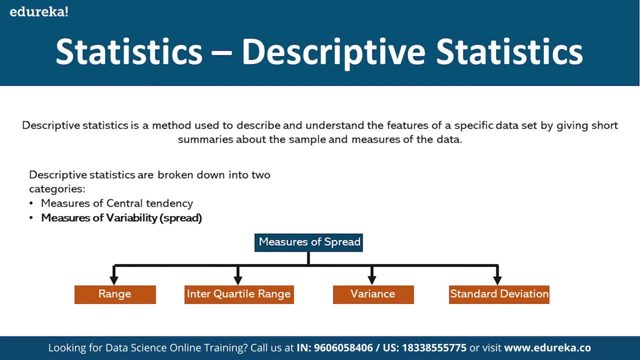 Variance means how data is varied from one to another. Standard deviation means how the data is deviated from the mean point. So these are the statistical terms which you need to be good at. So if you talk about measures of central tendency mean, 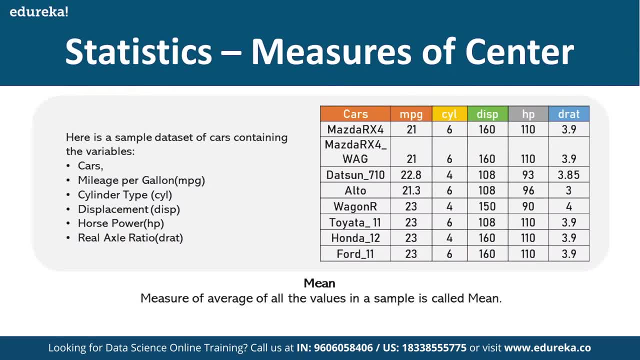 we already know. If you want to find the mean of a particular column, you sum all of them and divide by total number of elements. That is mean. So you might have seen average of a car. Like in every car, there is an average meter. 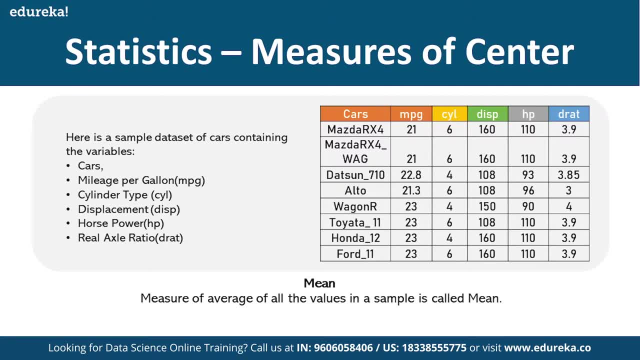 How it is doing. It is finding out how much kilometers you have driven for one liter of petrol or diesel And it gives you the average on the screen, which gets deviated all the time. So more of a- not in the older cars, but nowadays every car. 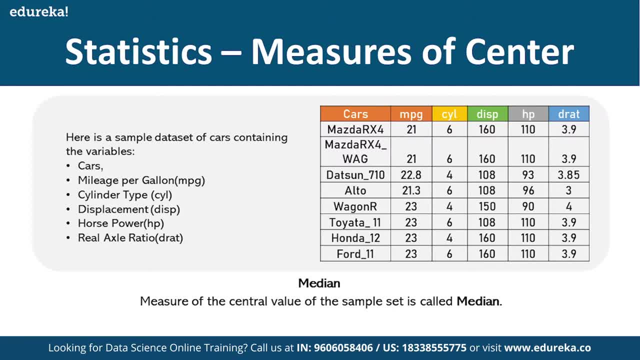 has that feature. finding the average Median is the middle value. If you sort the data in ascending, what is the middle value? Similarly, so this is a median Like if you talk about all this data, we sort it in ascending order. 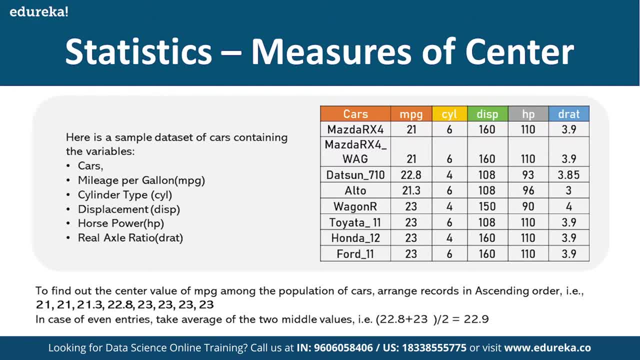 We take two middle values. take a sum of it. divide by two is the median. So here 22.8 and 23 are the middle values. When the number of elements are even, there are two middle values. We sum them and divide by two. That's a median. 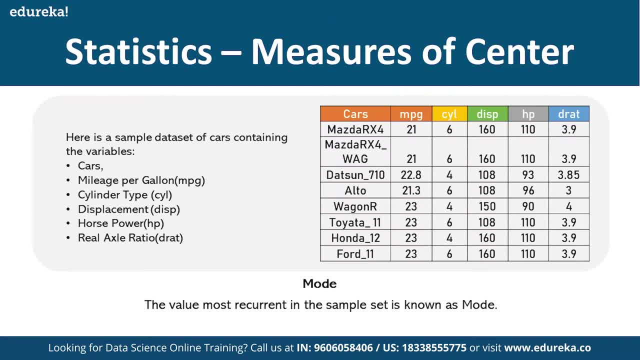 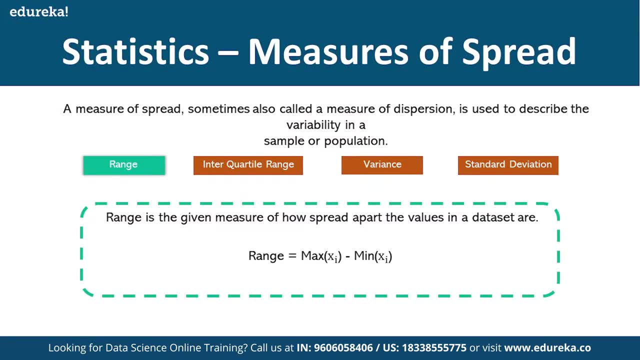 Similarly, mode is a maximum occurring value. So then the cylinder column 6 is a maximum occurring value. That is called as a mode. So if you talk about measure of speed, there is something called range Maximum to minimum. So range is maximum minus minimum. 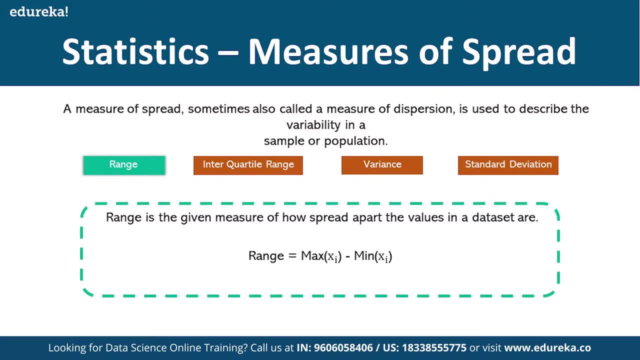 Suppose I want to see what is the range of speed of a car. So we have 0 to 200 kilometers per hour. That's a speedometer, That's a range of value a speed can attain. Speed can be attained Similarly, quartile. 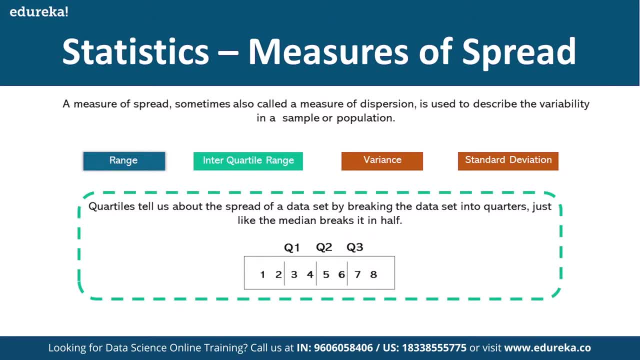 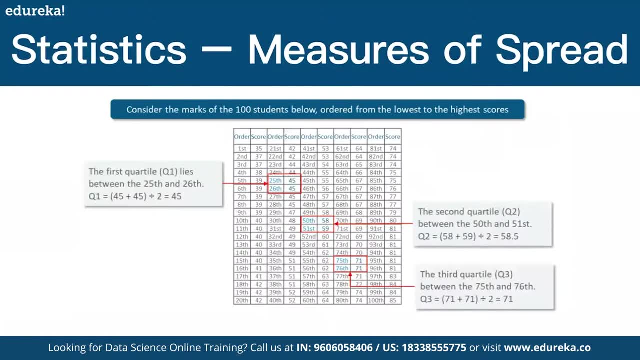 interquartile range, That is first quartile, second quartile, third quartile, 25%, 50%, 78%. that is known as a interquartile range. So here, first quartile is 45 and 45. 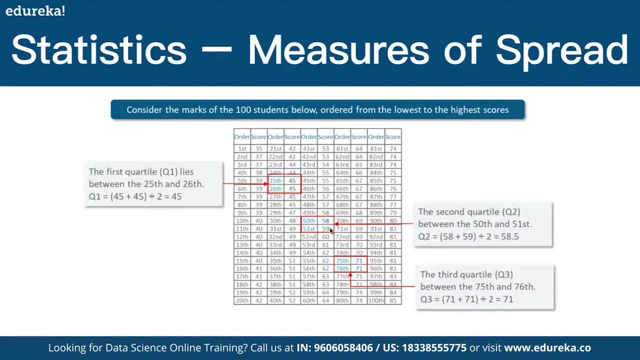 divided by 2 is 45.. Second quartile is 58 plus 59.. Third quartile is 71 plus 71 divided by 2.. So it is generally used in competitive exams. You might have seen percentile How you are performing as compared to other students. 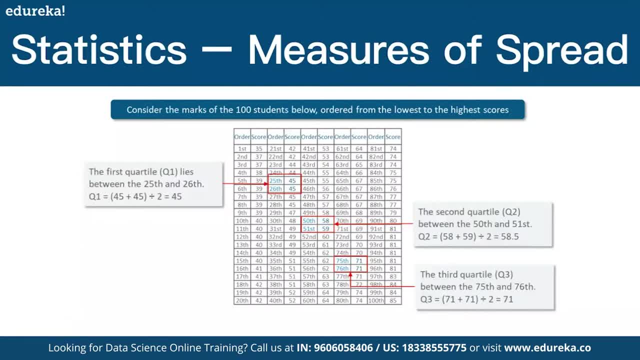 that's known as a percentile. Maybe student gets 40% marks in maths, but he has got 99 percentile Out of 100, a student can get 40 marks but his percentile can be 99 because 99 people are behind him. He is. 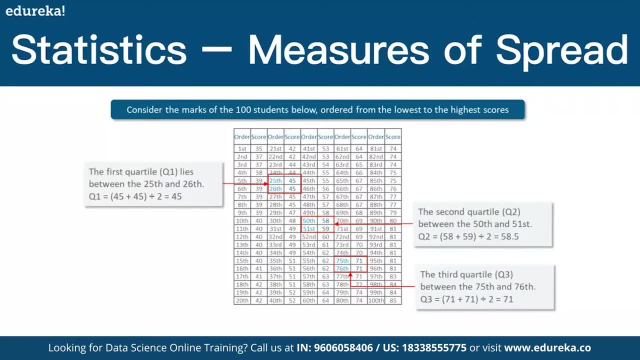 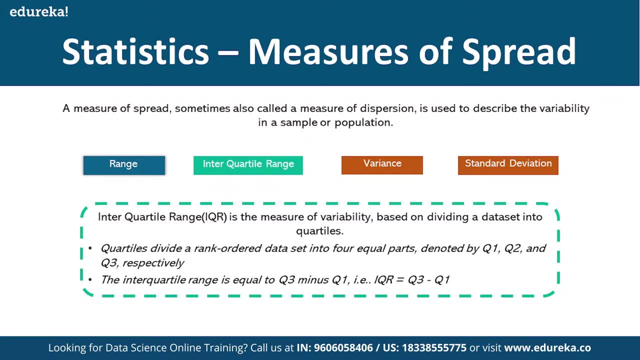 a topper of the class, All cut field. Similarly variance. So IQR method is finding- is used to find the outliers. I already told you IQR is another method. So there are four methods for finding outliers. One is IQR method. 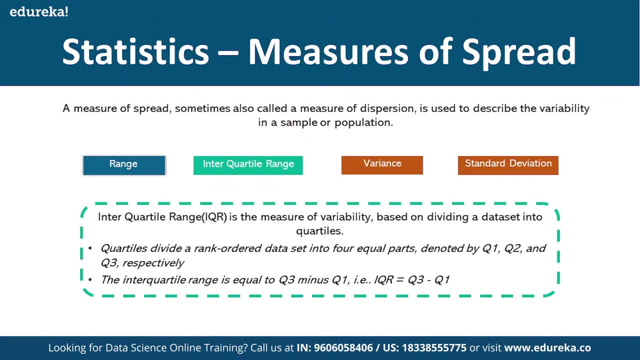 Another is three standard deviation technique, Third is Z score and fourth is box plot. If you want to note it down, there are four ways to find outliers: IQR method, three standard deviation technique, Z score and box plot. So interquartile range we have. 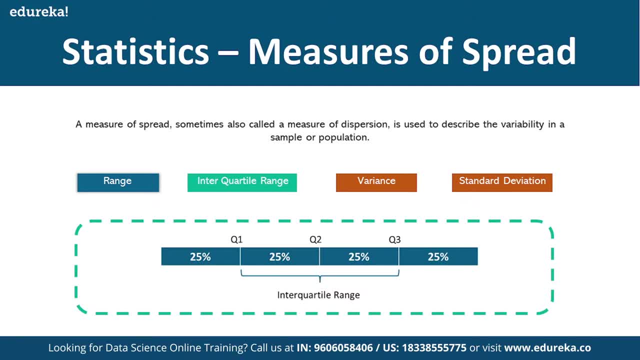 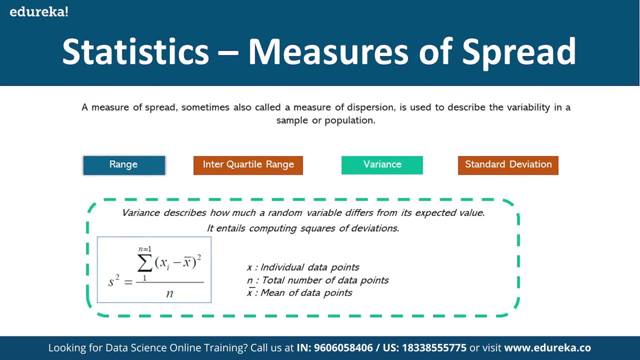 already discussed: First percentile, second percentile, second quartile, third quartile, 25,, 50 and 75%. Similarly, variance is difference from the mean. square it and sum it and divide by total number of elements. Formalize what. 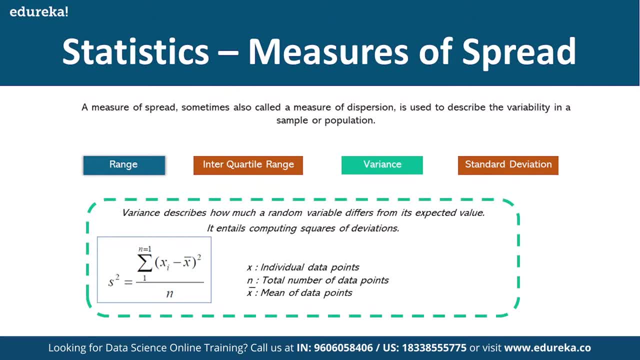 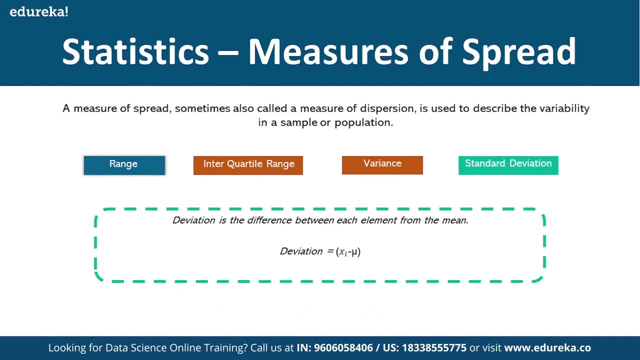 Subtract every value from a mean, square it and divide by total number of elements. Sum it and divide by total number of elements. That is known as variance. Standard deviation is mean minus deviation is difference of mean. each element from the mean. How much a value is divided? 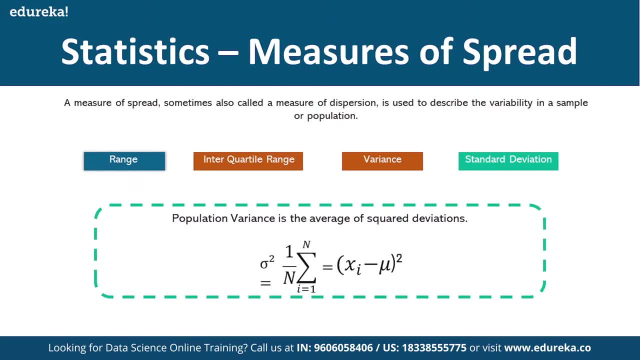 from the mean is known as standard deviation, And square root of variance is also known as standard deviation. Square root of variance is also known as standard deviation. So once you find variance, if you take a square root of it, it is called as standard deviation. 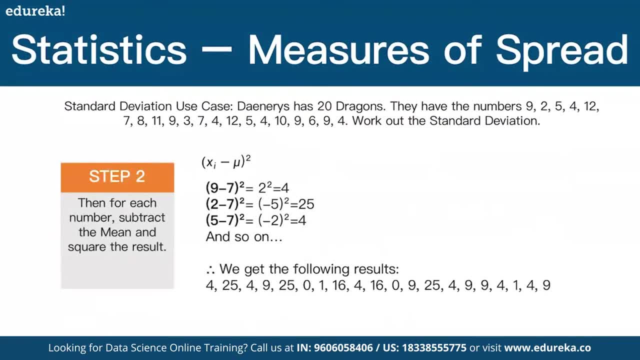 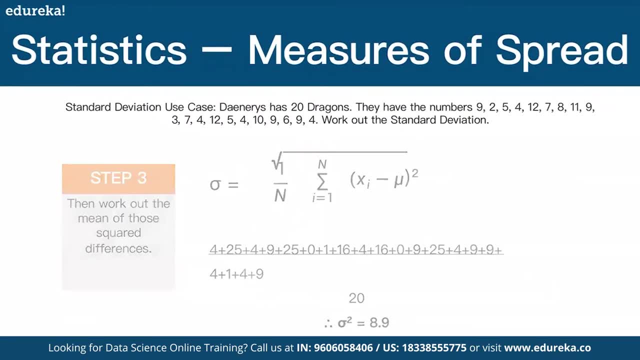 It is the same. So this is step by step. It is shown in the example how to find variance, how to find standard deviation using formula. But in Python we can directly get it done quickly with a direct function. suppose I will show you. 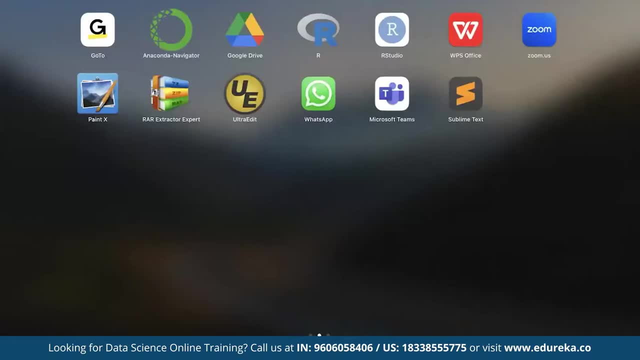 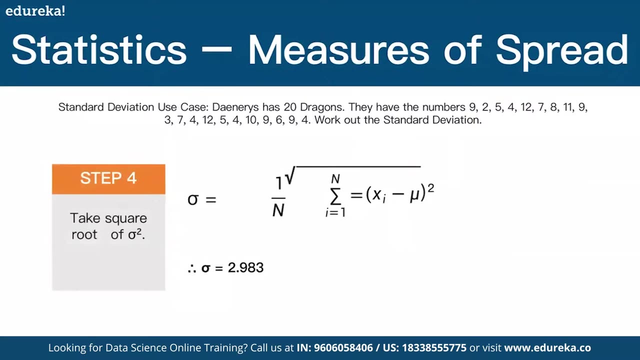 a small demo in Python. So in Python we have something called Anacondas Navigator, which is a tool on which we work on Python, And there is a tool in Anacondas called Jupyter Notebook. So you need to install Anacondas on your machine first. Anacondas is a 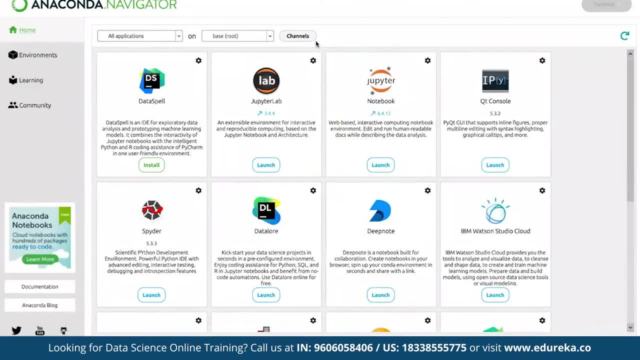 group of tools like MS Office. MS Office has Word, PowerPoint, Excel. Similarly, Anacondas has got multiple tools, like Spyder, Jupyter, Notebook. These are the tools comes with Anacondas. We need to launch Jupyter. It will create a notebook like we. 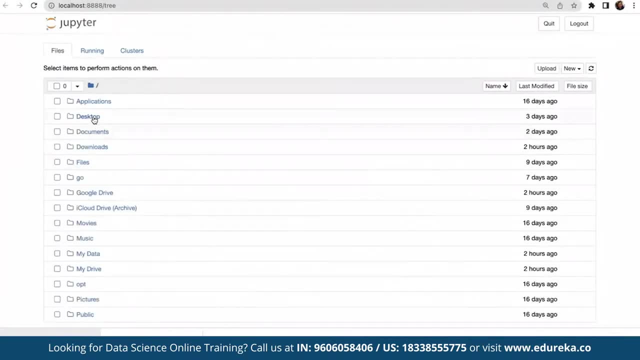 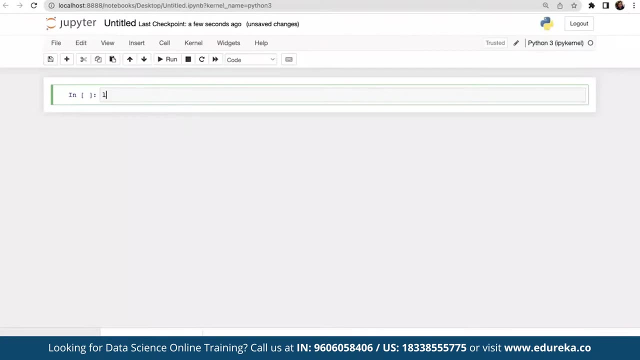 used to carry in our school days. And let's say, I go to desktop and create a new notebook, New Python 3 notebook, And I create a container, let's say a list, List one as let's say 2,, 3,, 4,. 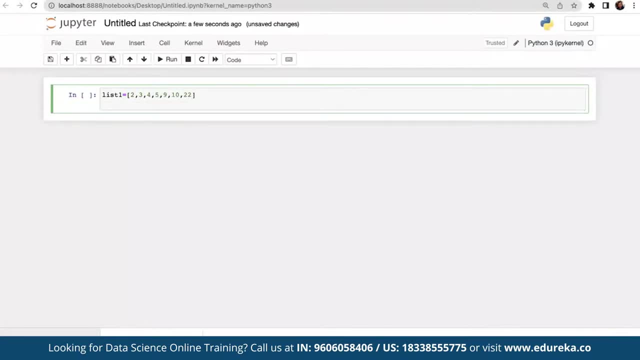 5,, 9,, 10,, 22.. And this is the container having multiple values And I import numpy And I will say numpyme mean of list one, We get 7.85 in one line. Similarly, if I say numpystandard deviation, 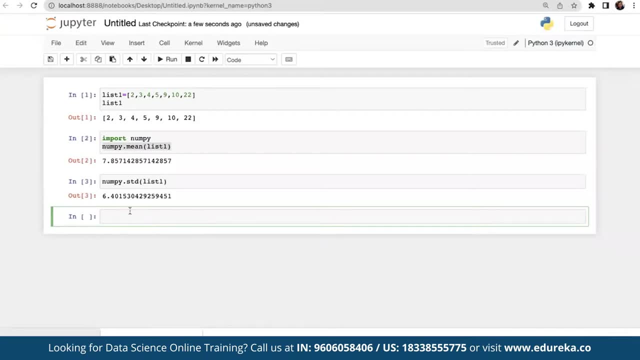 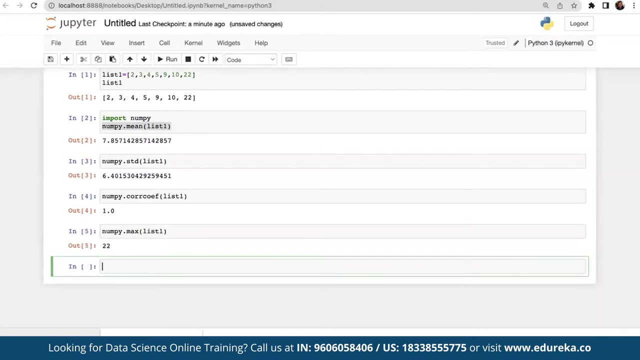 std, this is standard deviation, Right. If we say numpy correlation coefficient of list one In one line, you get one. numpymax, You get 22 as a maximum value. numpymin of list one: You get 2 as a minimum value. 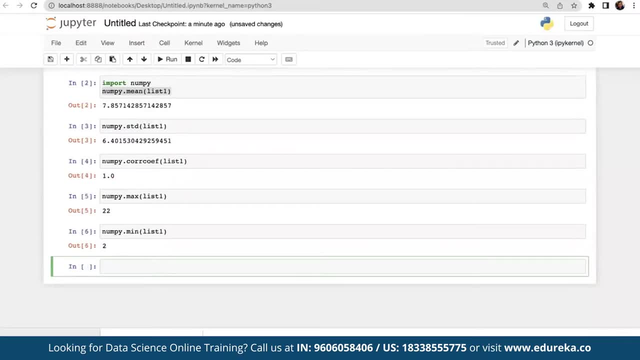 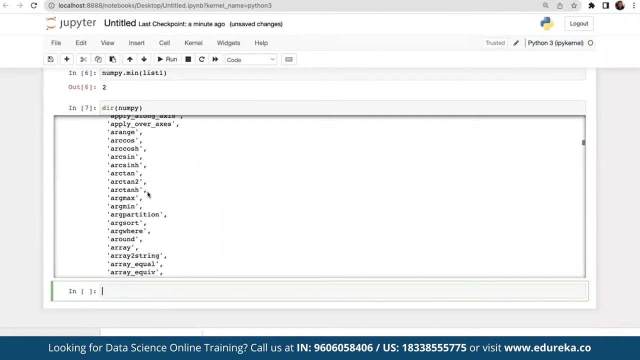 Right, So all these statistical functions are inbuilt in numpy. So if you see a dir of numpy, You will see all the functions in numpy. So many things are there. All the statistical and mathematical functions are there And mathematical functions are there in numpy. 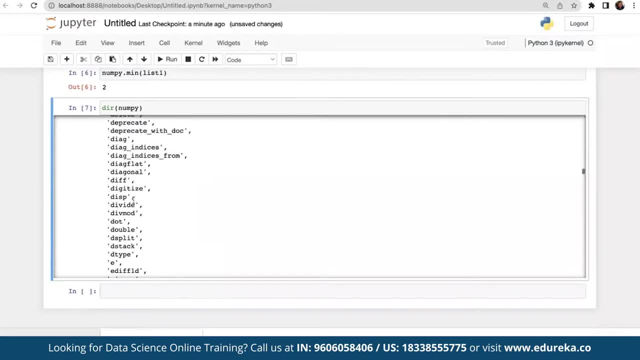 Cum sum Cumulative sum A lot of exponential Exp value, Absolute value. So many Hundreds of them are there For linear algebra. Log of 10.. Log to the base 2.. Similarly, if you import a math library, 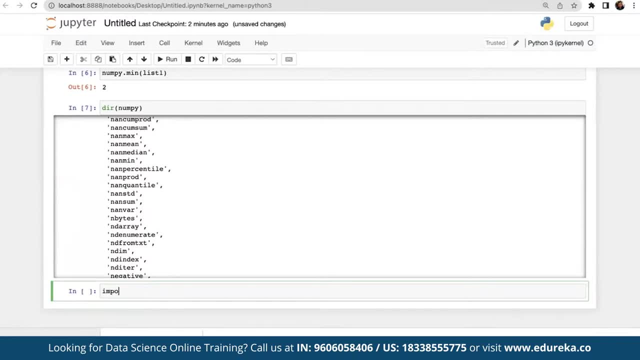 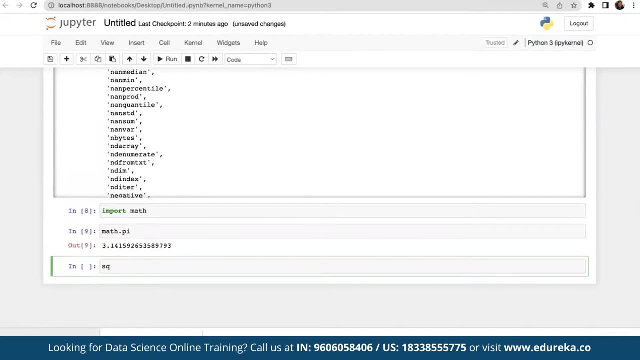 And you will say mathpi For a pi value. If you say sqrt, Mathsqrt Of 2. You get a square root value, Mathcosine Of 2 degrees, Mathpact Of 5.. So these are all inbuilt. 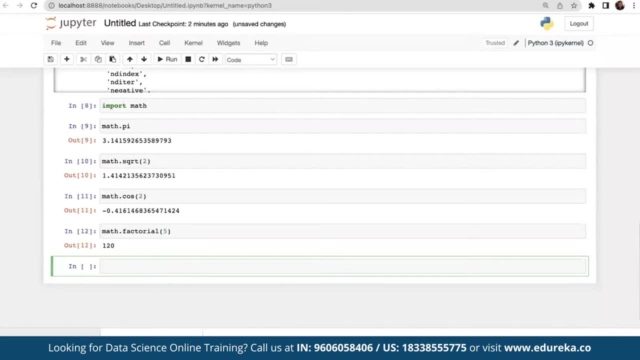 functions. in python You would have to reinvent the wheel, So you don't have to put the energy in writing the whole formulas for it. All these things are inbuilt. You just need to call the function, Pass the value And things are done.